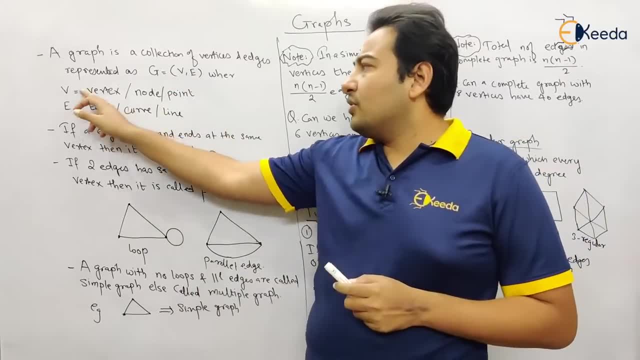 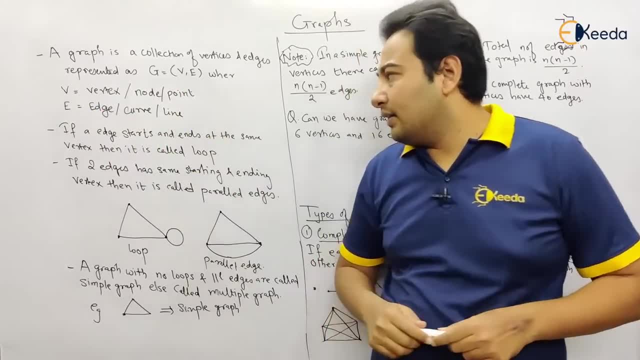 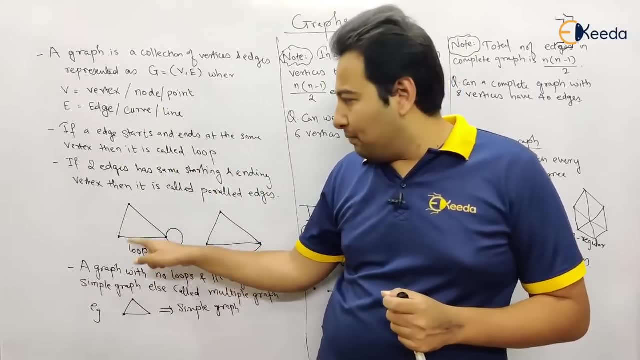 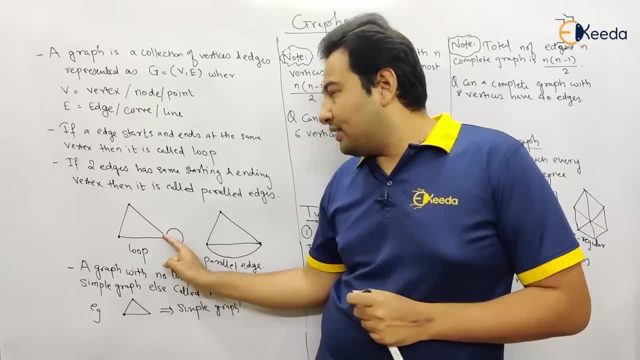 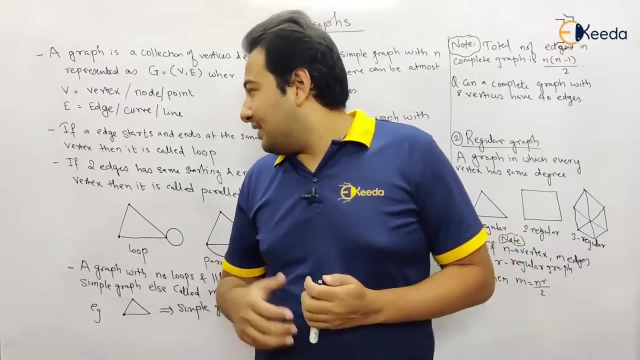 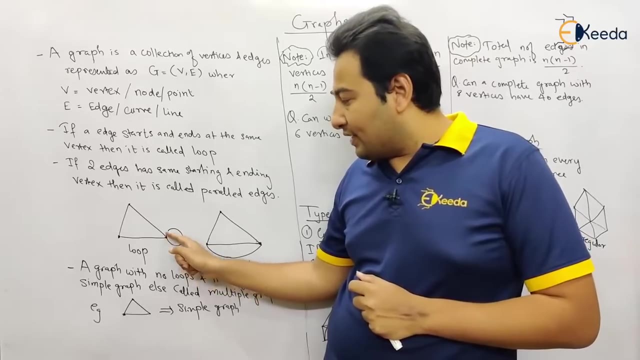 points. basically, These are the points and they are vertices, and these vertices are joined by lines that are also called edges. Next see, if we talk about this particular edge, it is starting and ending at the same vertex- Start, starting and ending at the same vertex- then it is called loop. and if there are two edges, 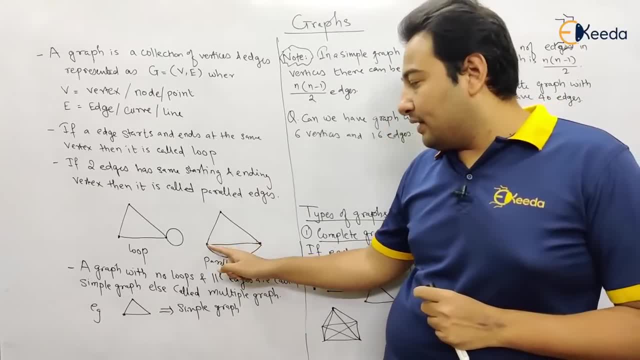 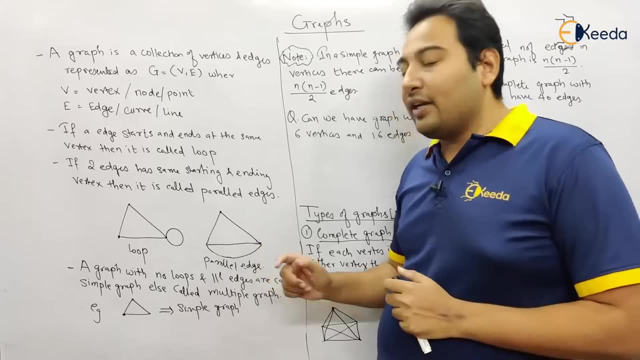 or two lines between the same vertices. here these two vertices are between these two edges are between these two vertices. they have same starting and ending vertex. then it is called parallel edges. so this is the example of loop, this is the example of parallel edges. so it's very important concept. 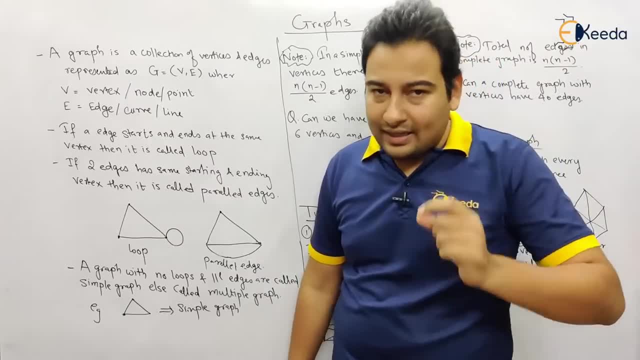 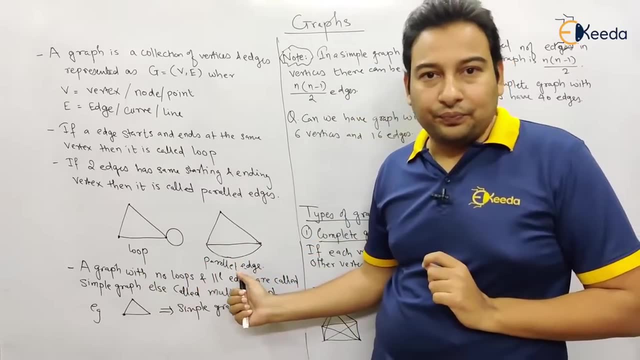 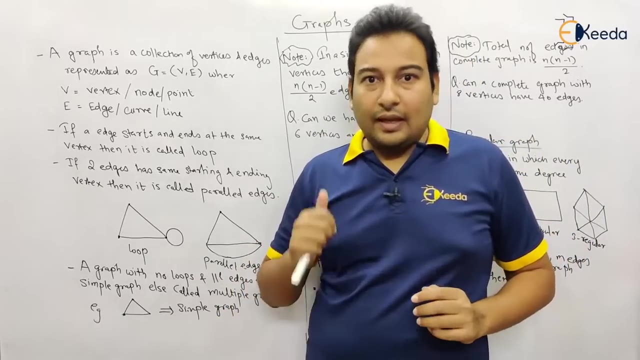 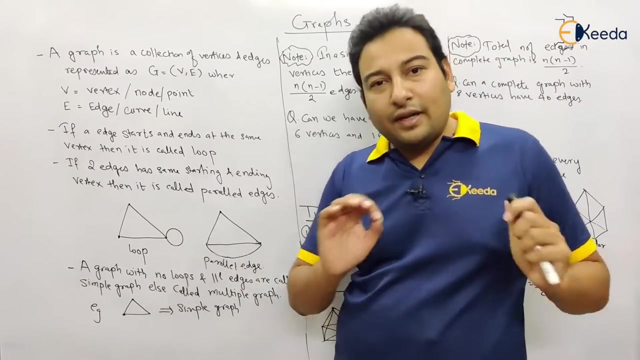 if a graph does not contain- listen to me very carefully- if does a. if a graph does not contain loop and parallel edges, does not contain loop and parallel edges, then it is called simple graph. if a graph contains loop and parallel edges, then it is called multiple graph. are you clear with the definition: simple graph and multiple graph? what is simple? 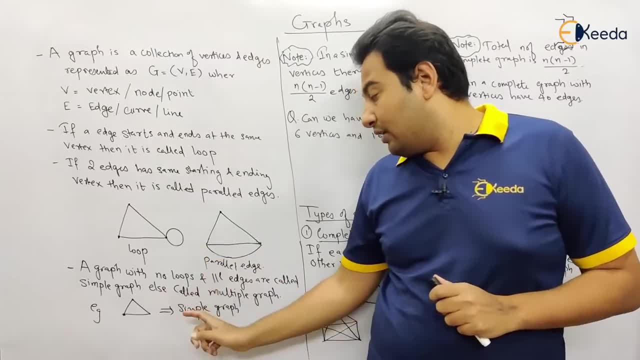 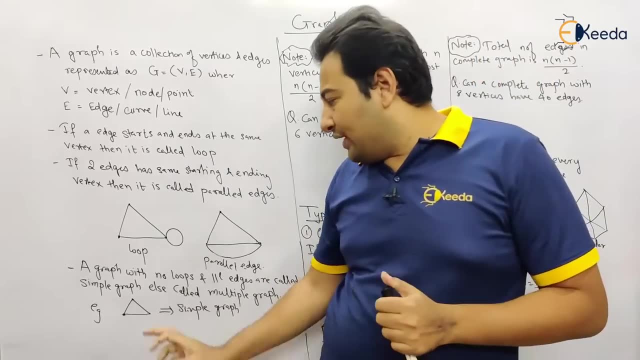 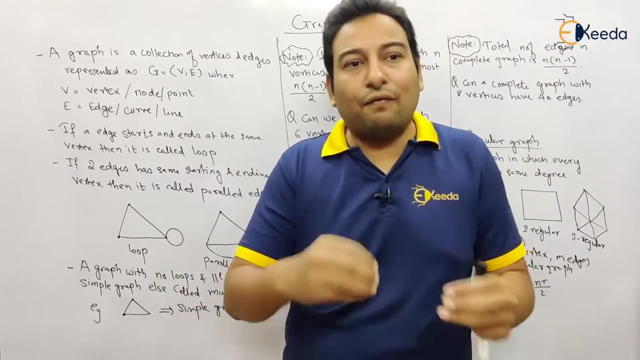 graph. it does not contain loop and parallel edges. and what is your multiple graph which contains loop and parallel edges? as far as our syllabus is concerned, we are going to study simple graph only. that means we not going to consider or we going to study those graph which does not contain loop and parallel edges. so what is the example of? 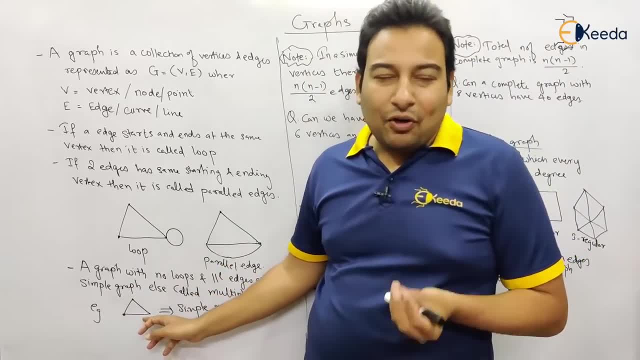 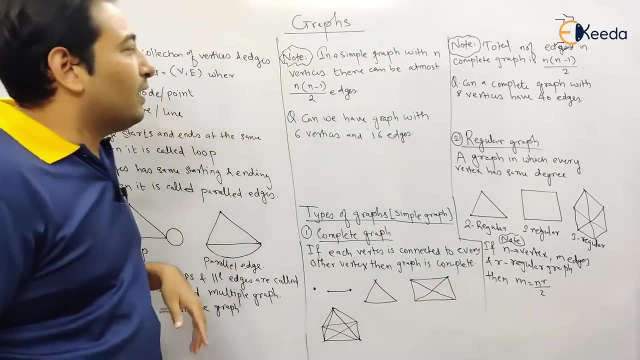 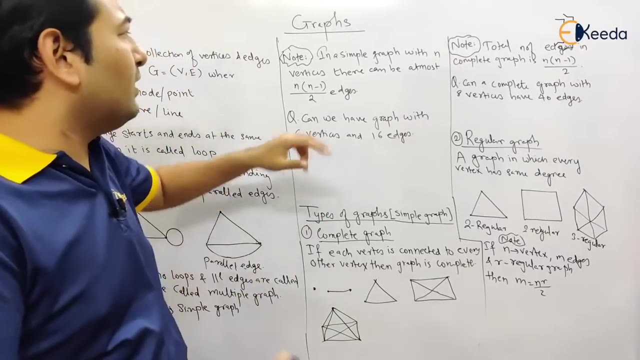 simple graph. see this: this is an example of simple graph. where is where there is no parallel edge, as well as there is no loop. let us move on. let us discuss a very important concept, which is important. point note: you can get a question on this in the exam- mcq gate or so on- in a simple 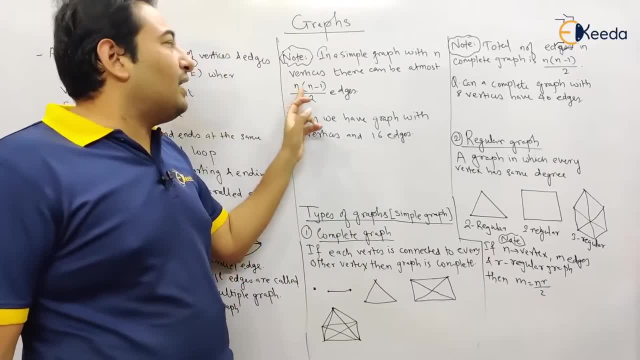 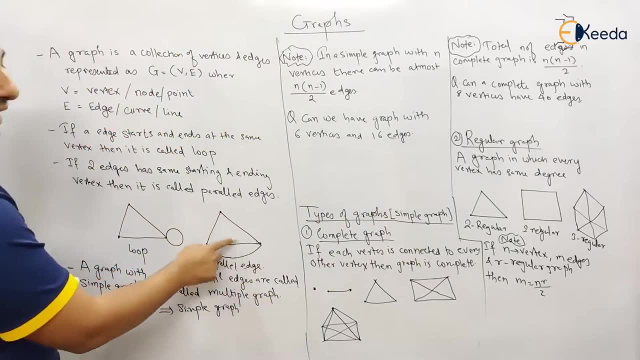 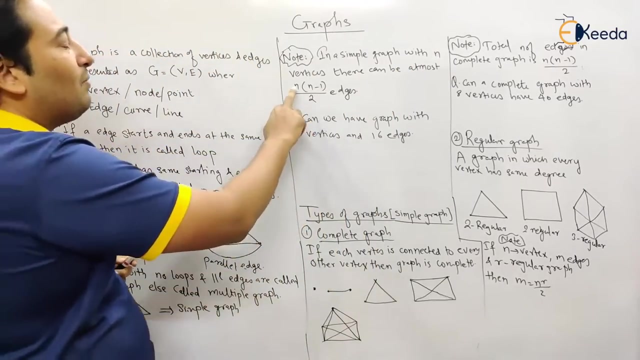 graph. with n vertices there can be at most n into n minus 1 upon 2 edges. first of all, it's a simple graph. simple graph means there is no loop as well as parallel edges. so if this is the case, if n vertices are there, there can be maximum n into n minus 1 upon 2 edges. for example, 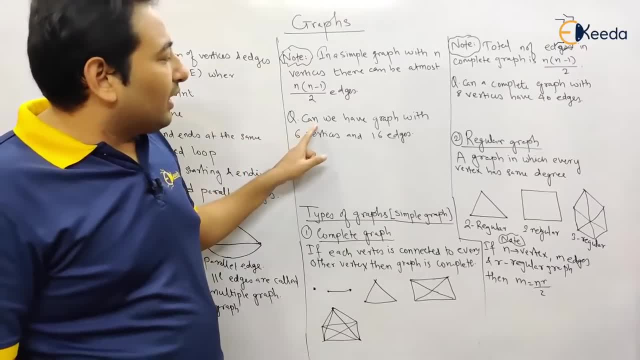 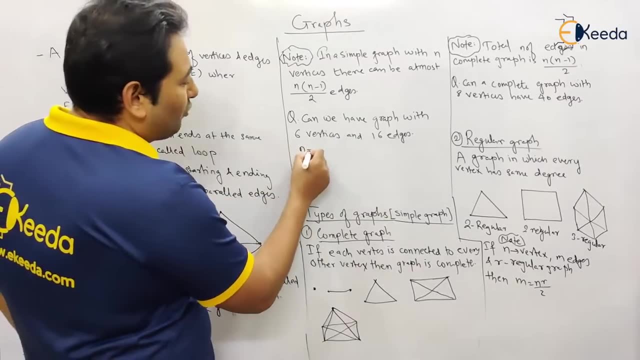 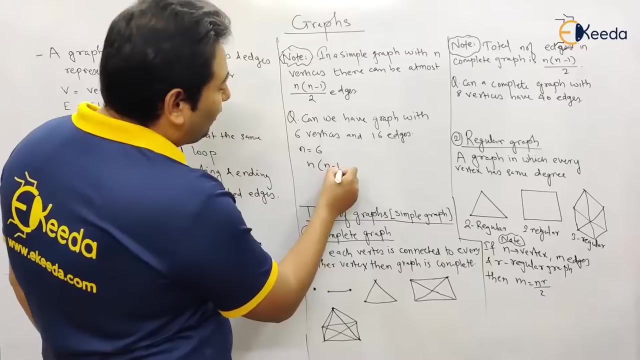 a question is asked in previous lecture. if you have a question, you can ask a question in previous paper. can we have graph with 6 vertices and 16 edges? how many vertices are there? n is equal to 6. how many at most maximum? how many edges are possible? n into n minus 1 upon 2. 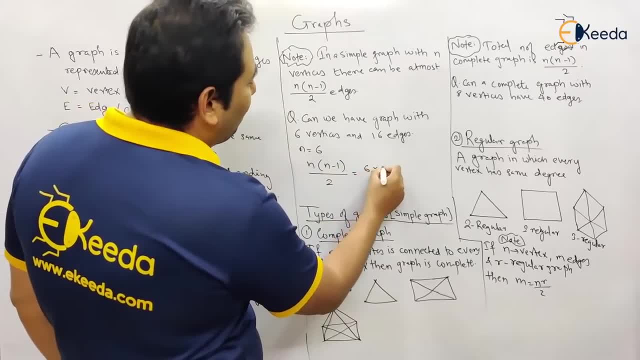 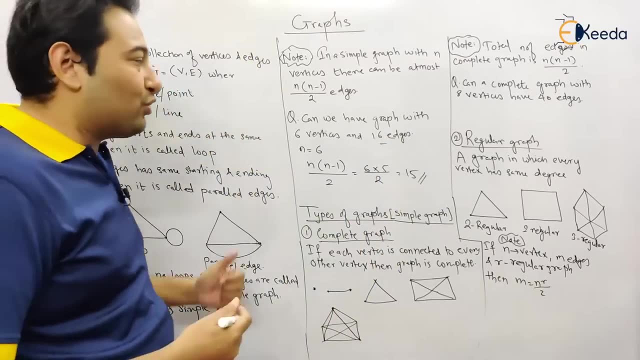 so if you take n is equal to 6, so this will become 6 into 5 upon 2, so that is 15 and it's saying 16 edges. so it is possible. no, it's not possible. if a graph has 6 vertices, then it's. 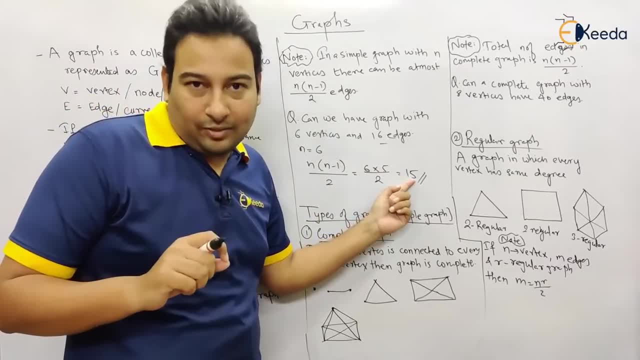 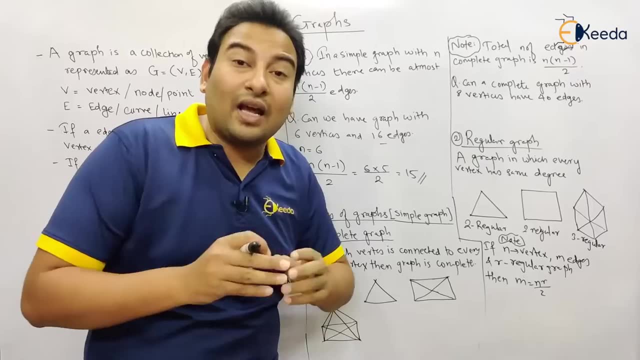 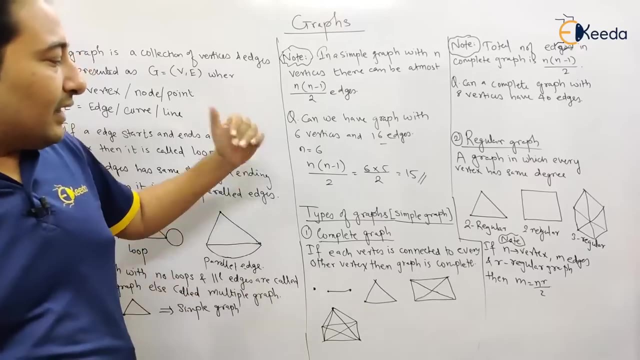 10. it can maximum have 15 edges. now see nowhere in the problem. it is mentioned simple graph, but by default throughout the chapter chapter. whenever i talk about graph, it's by default a simple graph. is this clear? so it's not possible. next types of graph. now we'll see what are the different types. 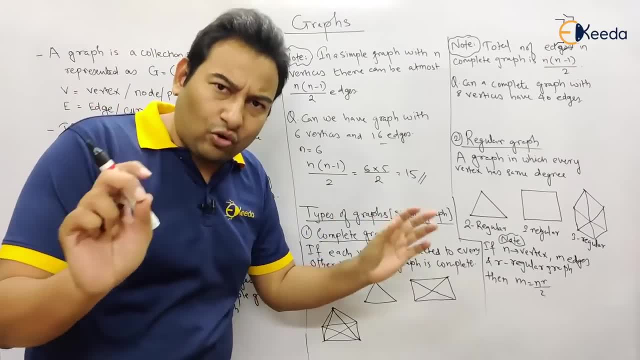 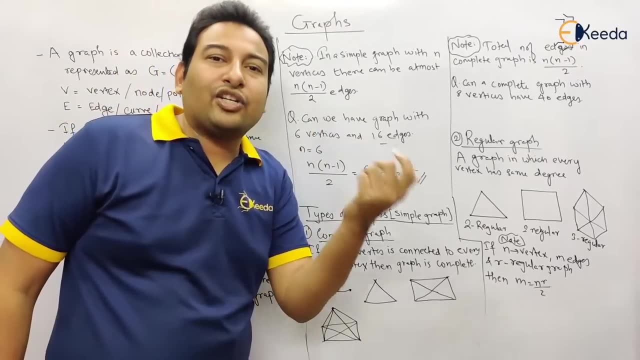 of graph, first of all types of graph, or you can say: simple graph, because we are talking about simple graph, only complete graph. what do you mean by complete graph? if every vertex is connected to every other vertex, then it is called a complete graph. see here, here there is only one. 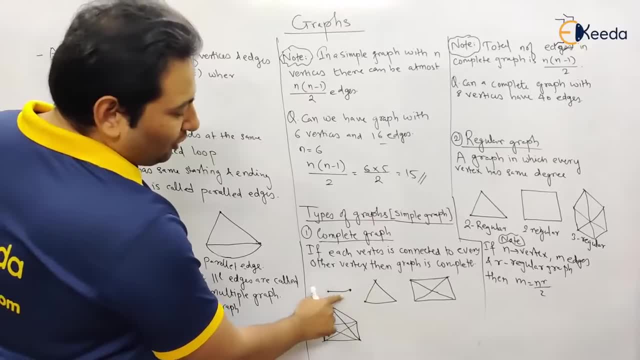 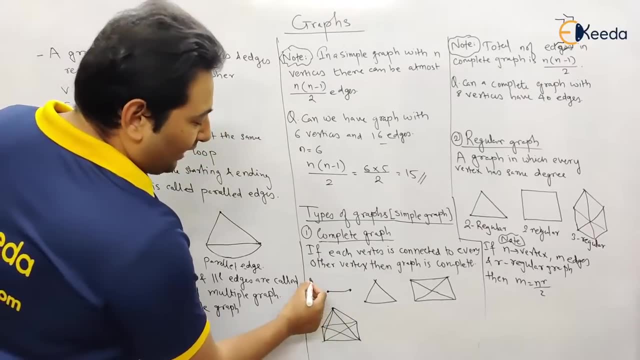 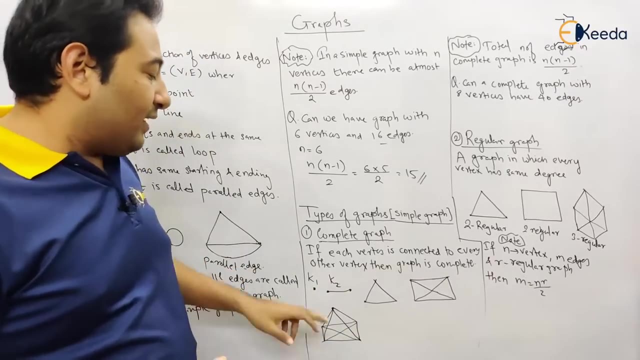 one vertex, so no need to think about it. if we talk about this particular graph, see, there are only two vertices and they are connected to each other. see, they are connected to each other actually. this is k1, this is k2. a complete graph is represented with, basically, km. you can say where 2 is or kn. 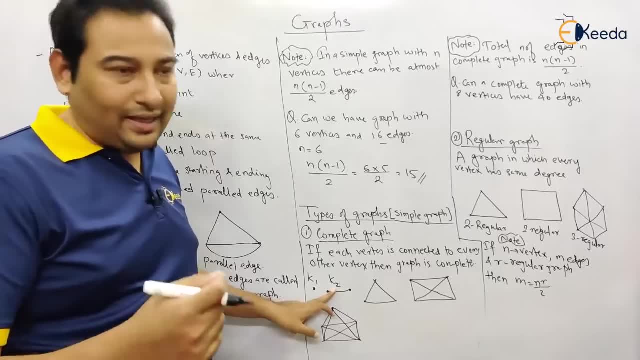 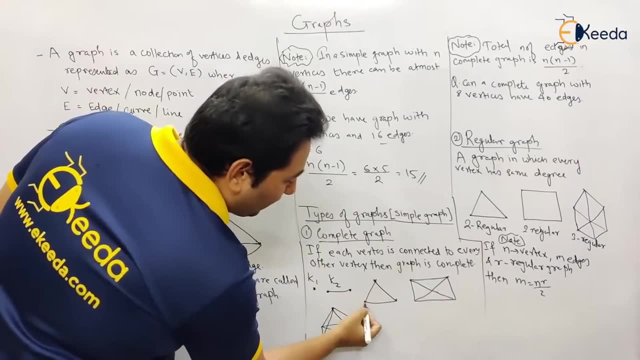 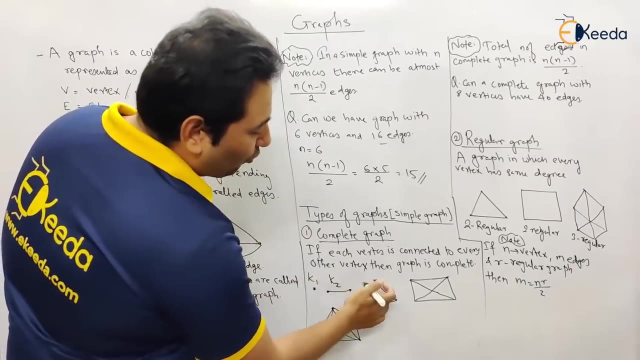 basically kn, not km. kn. n is what number of vertices. so, since there are two vertices, therefore it is k2. what about this? see this is also complete graph why there are three vertices and all are connected to each other. see here, this vertex is connected to this, this, this is connected to both and this is also connected to both. therefore it is k3. k3 means. 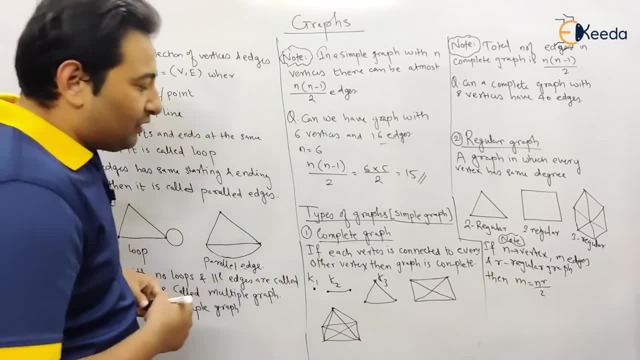 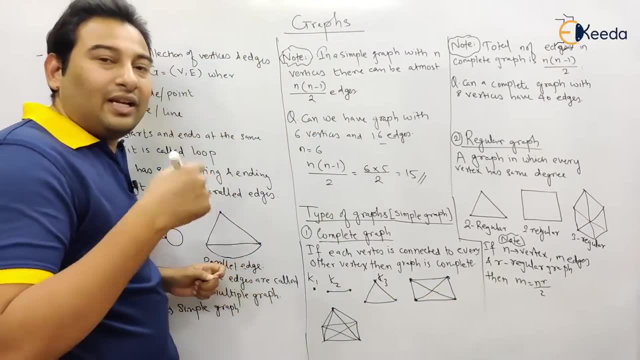 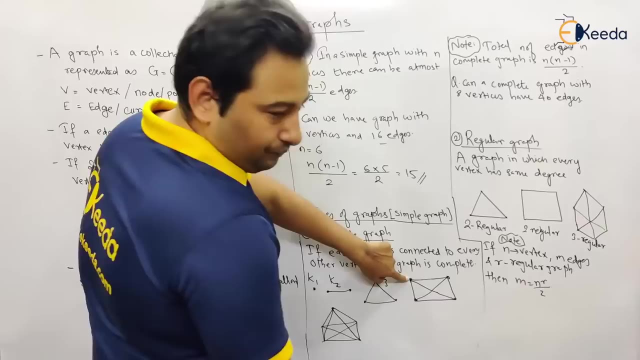 there are three vertices. therefore, it's a complete graph of k3. next, what about this graph? is it a complete graph? let us check each vertex should should connected to other vertex of the graph. see, this vertex is connected to this, this and this. that means this is connected to remaining all the. 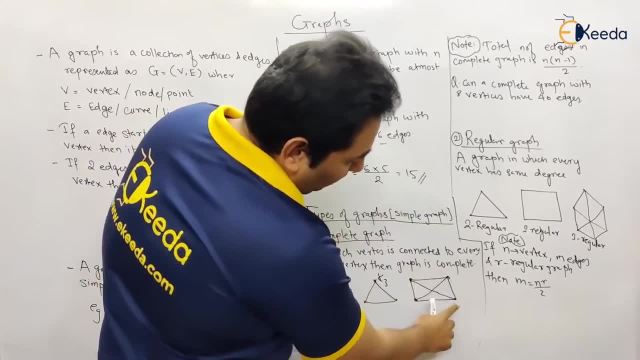 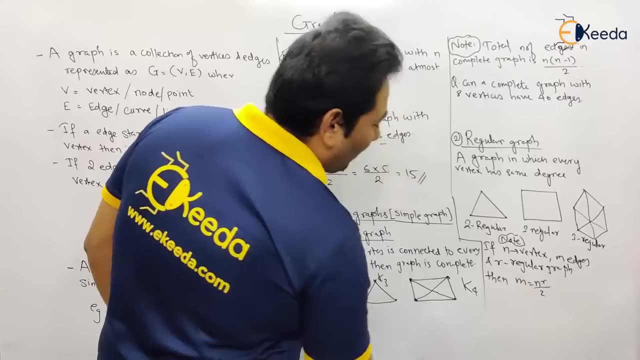 vertices. what about this? again the same story. see here. if you talk about this, again the same story. and if you talk about this, again the same story, that means this is also complete graph and since there are four vertices, therefore, it will be k4. what about this? this is k5. check. see this. this is. 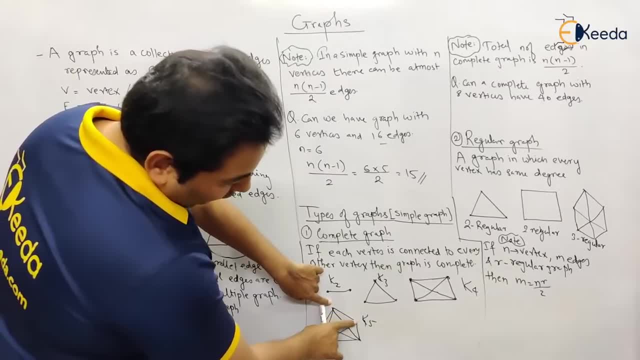 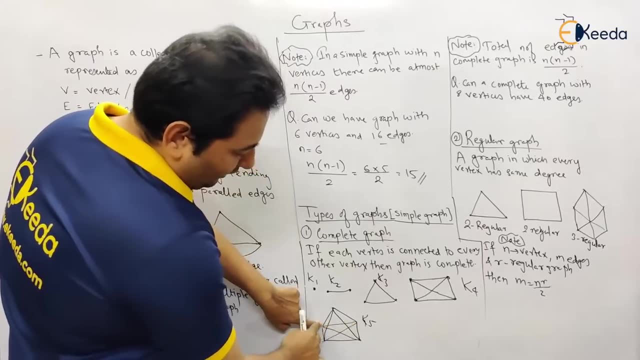 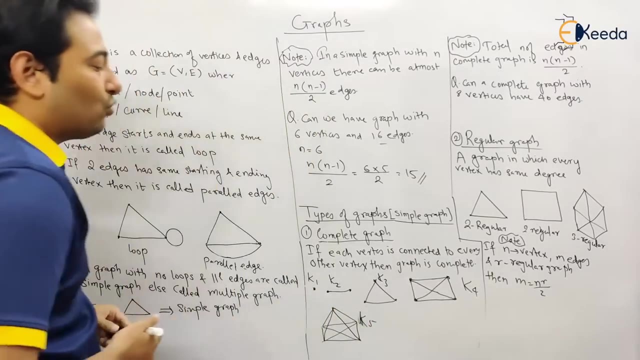 connected to this. this direct connection should be there. see, if we talk about this, let us check. it is connected to this vertex, this vertex, this vertex and this vertex. now you can check. each vertex is connected to all the remaining vertices. therefore, it is called a complete graph and it is represented. 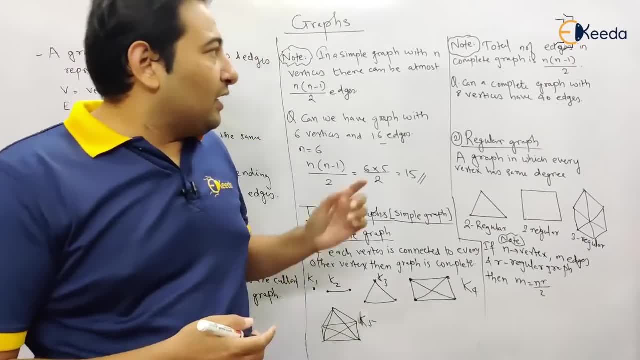 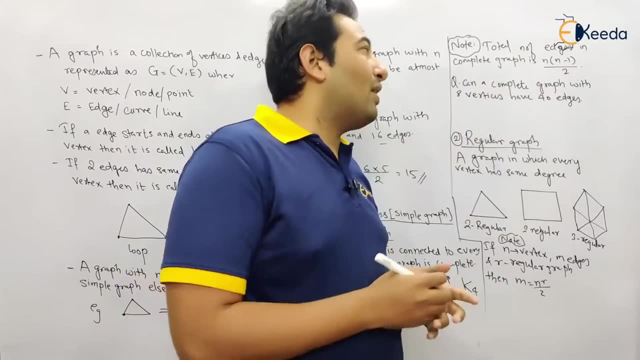 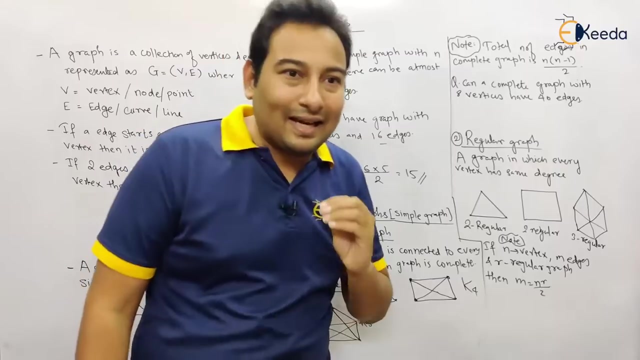 by kn, where n is your number of vertices. let us move on now. there is a point again. total number of edges in a complete graph is n into n minus 1 upon 2.. see, first of all, we are talking about the simple graph. we are talking about the simple graph. simple graph means: 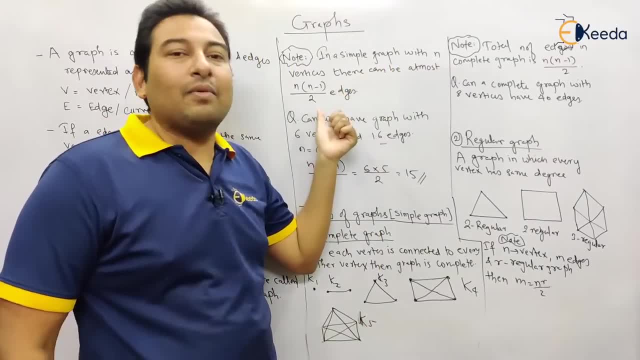 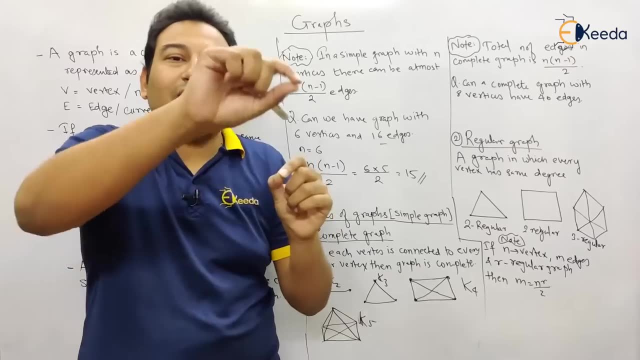 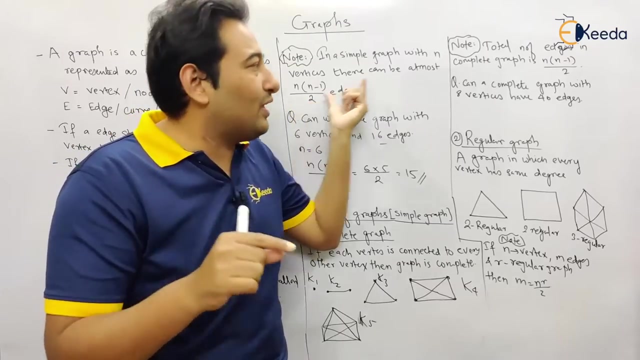 if there are n vertices, maximum, there can be n into n minus 1 upon 2 edges. right now, what do you in my complete graph? complete graph means every vertex is connected to every other vertex. that means in that case. so here the maximum possibility is what? n into n minus 1 upon 2. so that is the. 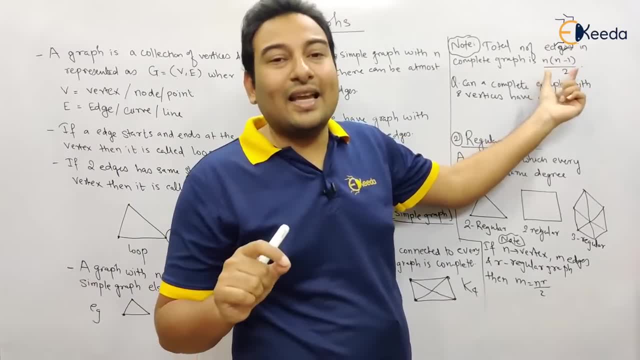 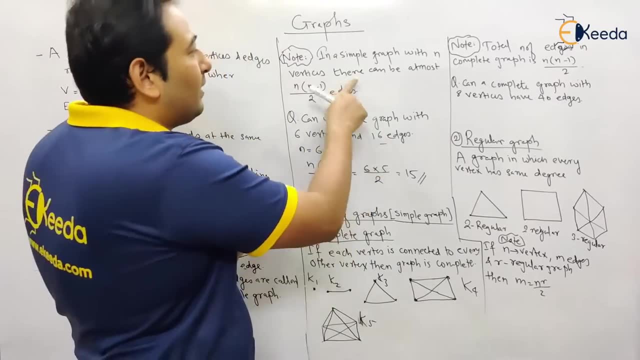 result. so in a complete graph, n vertices n into n minus 1 upon 2 are number of edges. is this clear? because, see, the maximum possibility in the simple graph is n vertices n minus 1 upon 2. these are the edges and this is the maximum possibility which is satisfied in the complete 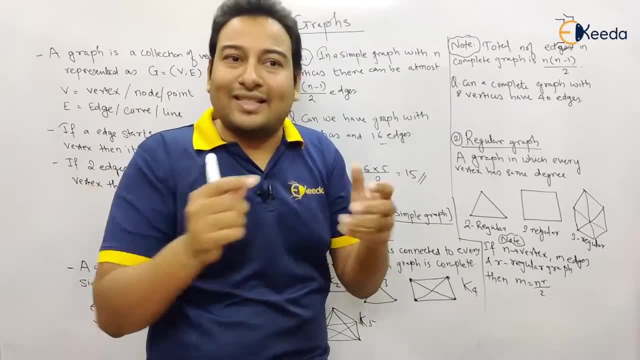 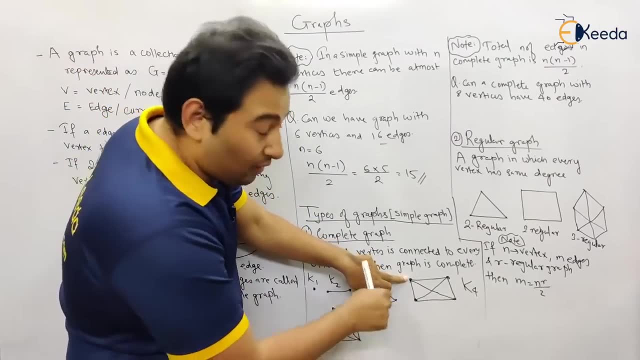 graph, because in complete graph, every vertex is connected to every other vertex. that is the maximum possibility. see, here there cannot be more, uh, more than these vertices, more edges, because, see, every age is connected to every vertex, is connected to every other vertex. that means all the possible. 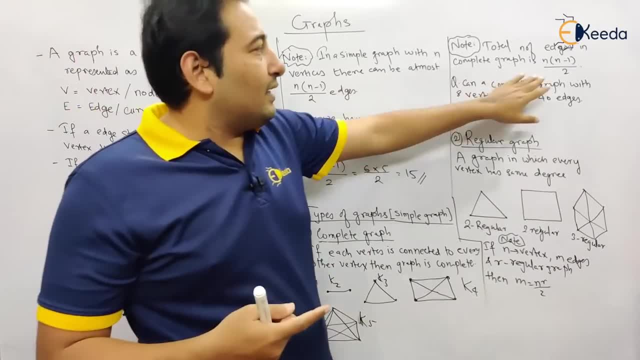 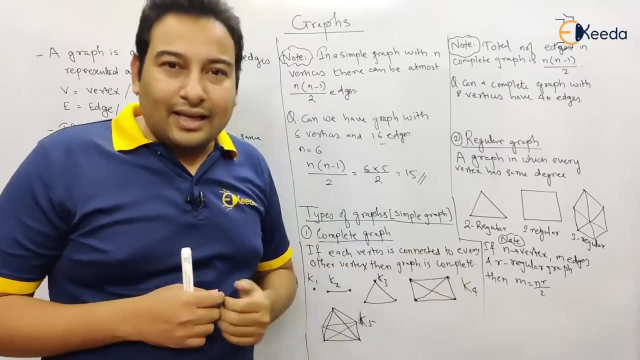 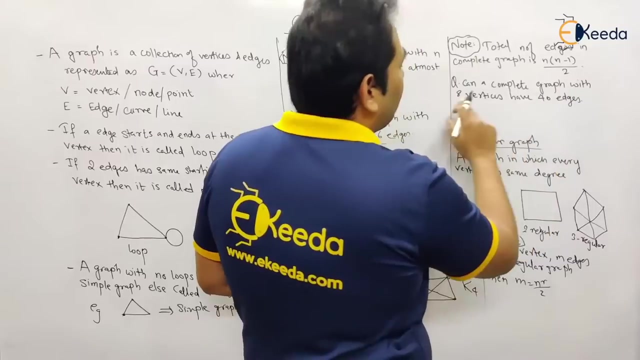 edges, or in short, here the utmost case is you can say the only case here. so if it is asked to find it is the number of edges in a complete graph, you just need to use this formula. for example: here it is given can. a complete graph with eight vertices are 40 edges. here the vertices are eight. 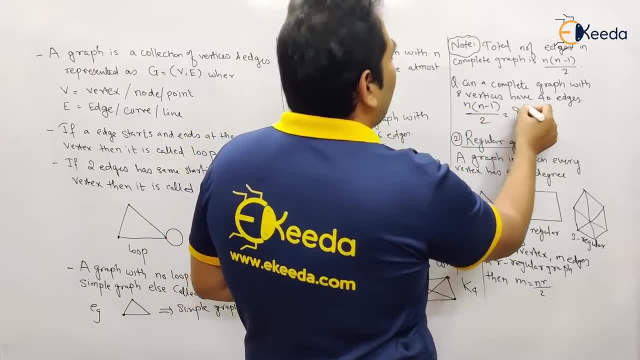 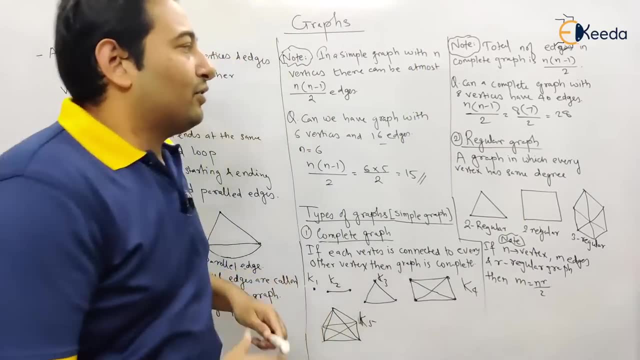 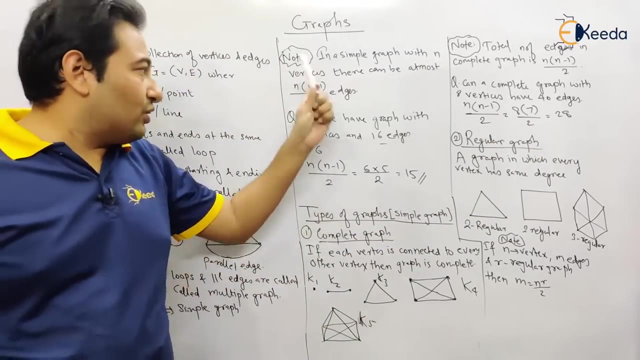 so it is n? n minus 1 upon 2. so 8, 7 upon 2. so that is what? 28. so it can it have 40 edges? no, because maximum edges it can have is 28. so let us move on. so this is what about complete graph. next type of: 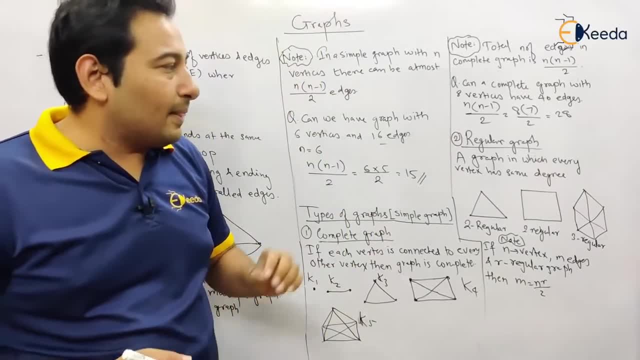 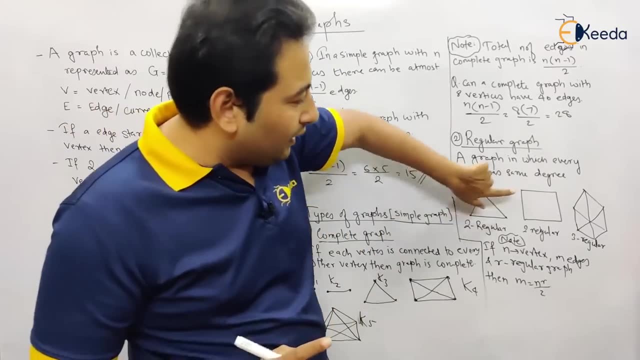 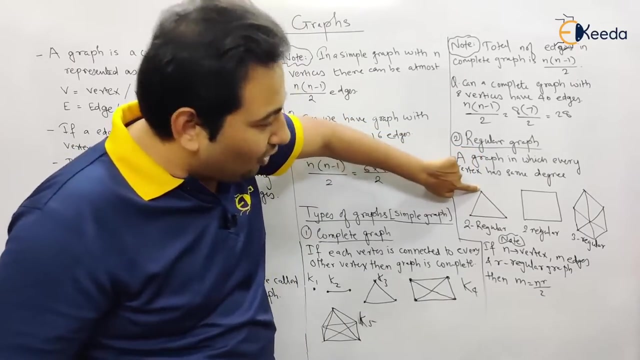 graph is called regular graph. regular graph means each graph must have same degree. what do you mean by degree? first of all, see here, if you talk about this particular vertex, how many edges are connected to that vertex is a degree. if we talk about this particular vertex, there are two edges connected. 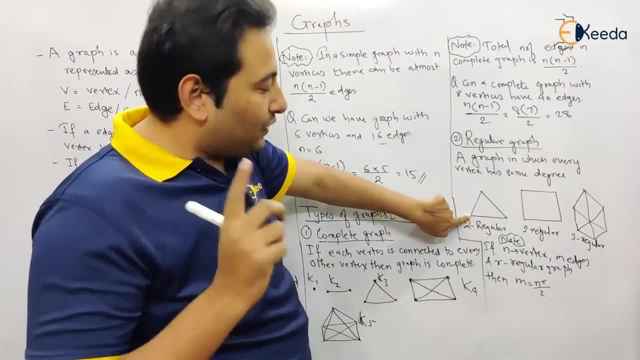 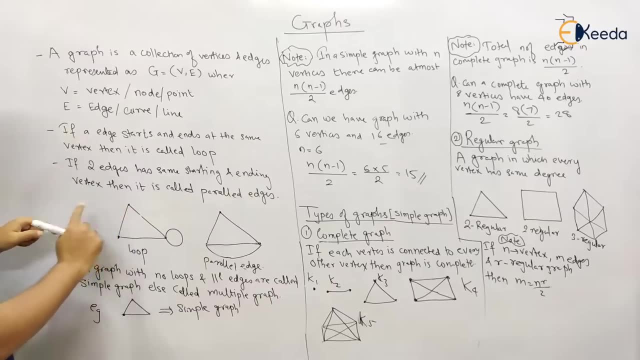 therefore, vertex of this degree is two vertices of this degree, is two vertices of these degrees. two: let us talk about, uh, let's say random. let's say what is the vertex of this degree? again, two: what is the vertex of this degree? how many edges are connected? one, two and three, so that 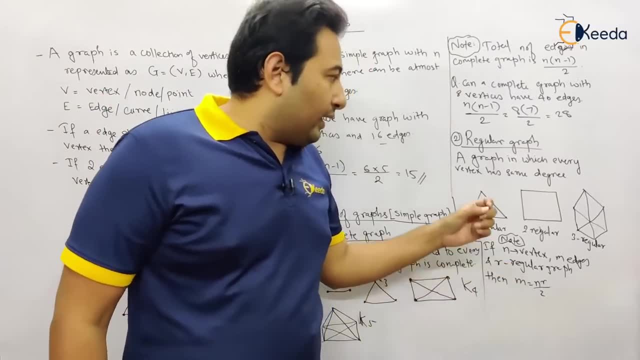 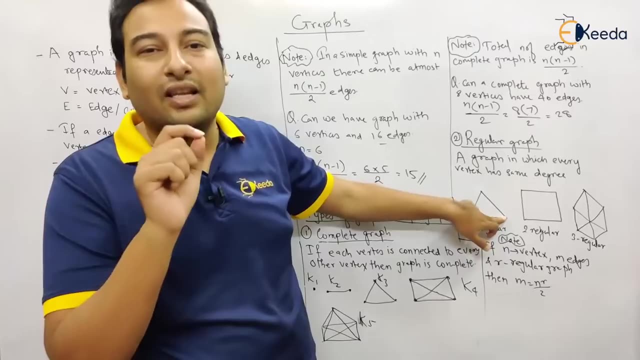 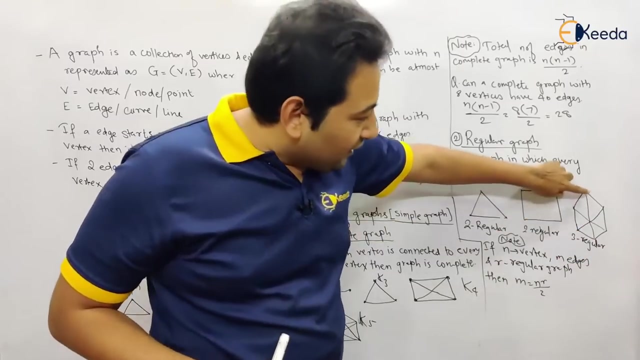 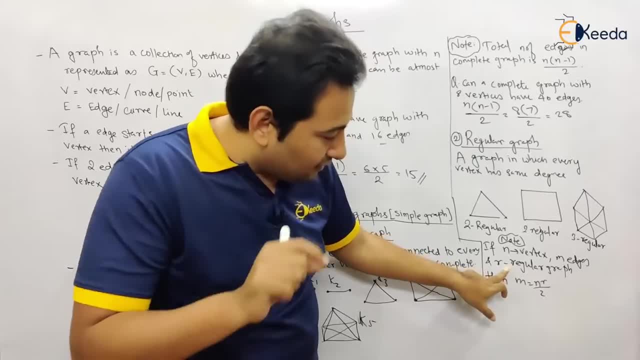 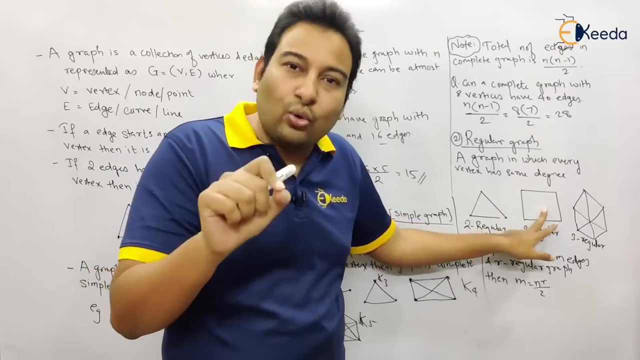 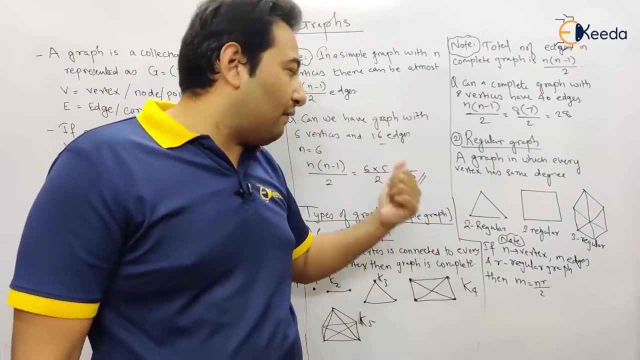 connected as r, c, r slash regular graph. that means this is two regular graph. why? because every vertex has degree two. this is also two regular graph. this is three regular graph. so are is this difference clear between the complete graph and the regular graph? so what you, what can, what you? 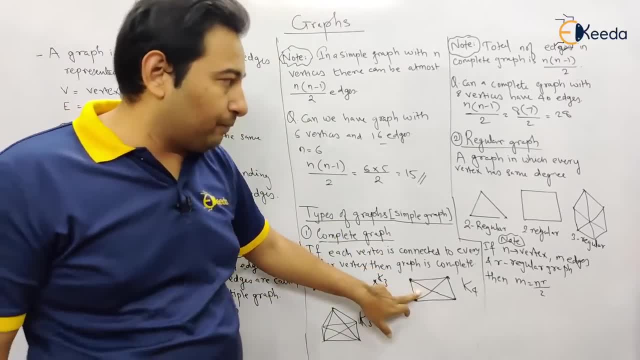 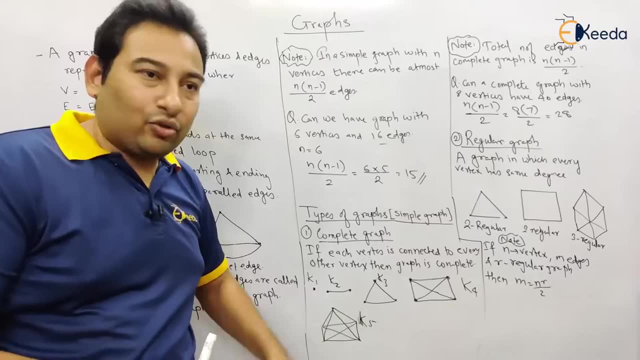 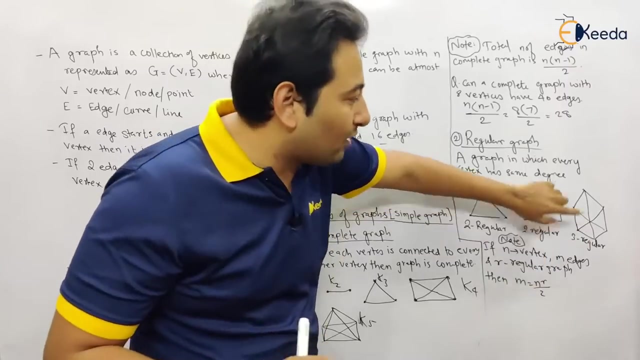 can conclude is every graph which is a complete it has to be regular. see, here it's a regular graph. why? because every uh vertex has the same degree. so every graph which is a complete is a regular, but vice versa is not true. this is regular, but it is not complete. why not complete c? this vertex is connected to this. 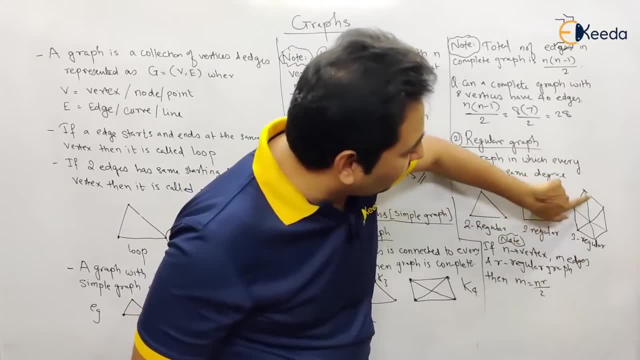 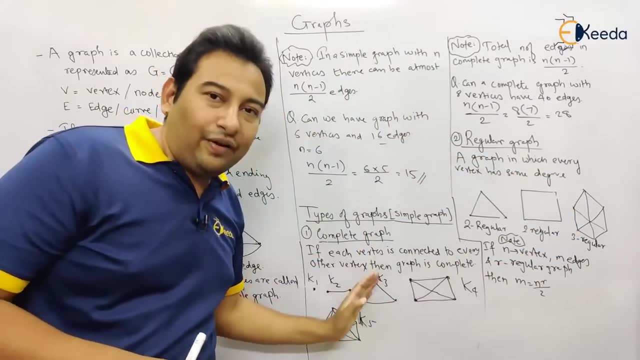 it is connected to this. it is connected to this. there is no connection between this vertex and this vertex. indirect connection we don't want, we want. we want direct connection. so what is the conclusion? if it is complete, then it is regular, but if it is regular vice versa is not always. 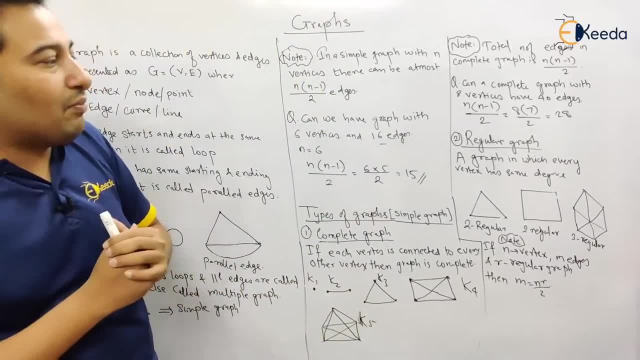 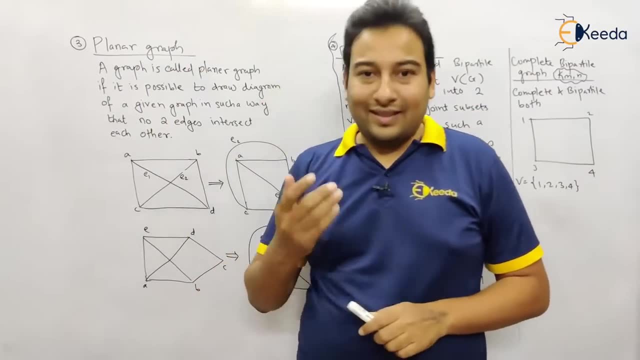 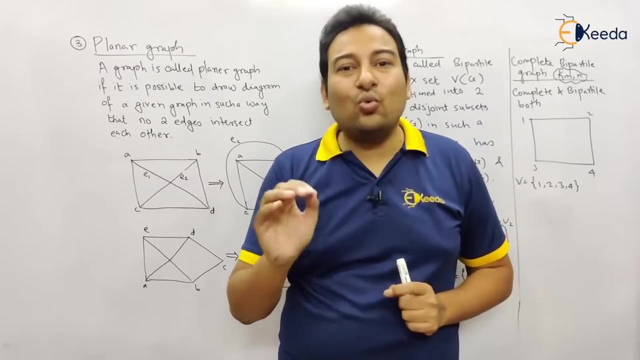 true, are you clear with this? so this is your tie type number two- regular graph. let us talk about the next graph, that is planar graph type number three. you can say it's very simple what the planar graph says. there should not be any two edges that. 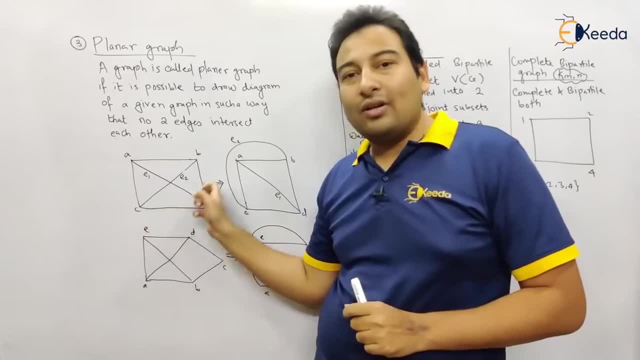 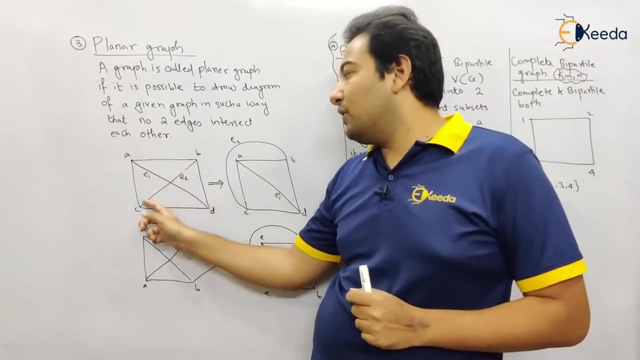 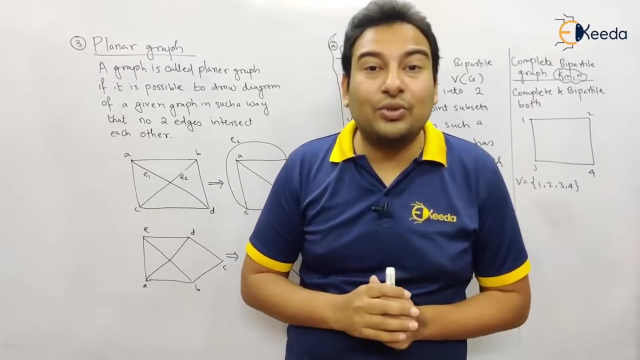 is intersecting each other. see here: what about planar? is it a planar graph or not? what is the rule? there should not be any two edges which intersect each other. now, if you observe these two edges, they are intersecting each other. so the rule says there should not be two edges which is intersecting each other. but 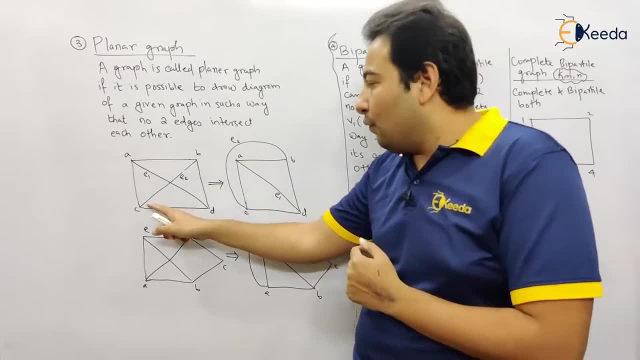 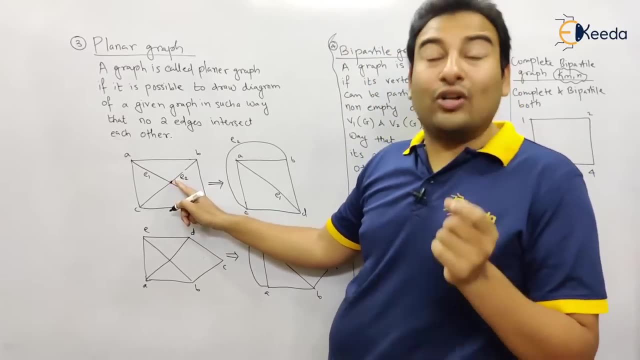 this graph can be redrawn in this way where the h, b, c, actually they are not intersecting, because see if, if there is no connection here, if there is a point or there is a vertex here, then you can say they are intersecting. this particular graph you can redraw in a such a. 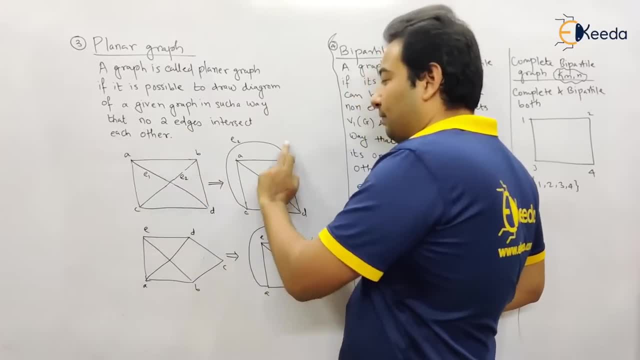 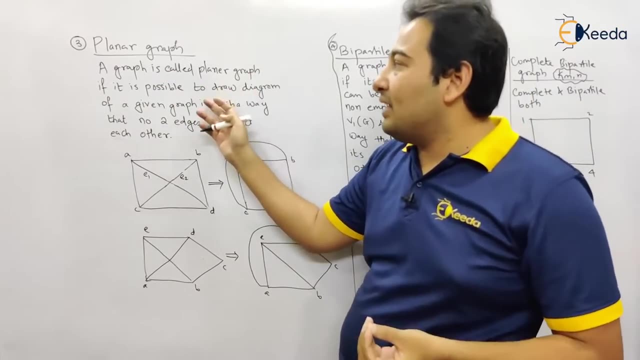 way that. see b c. you can redraw b c. now you can say no, two edges are intersecting each other. then the graph becomes planar graph. the definite edge becomes flat and the edge details are intersecting. definition is a graph is called planar graph if it is possible to draw diagram of a given graph. 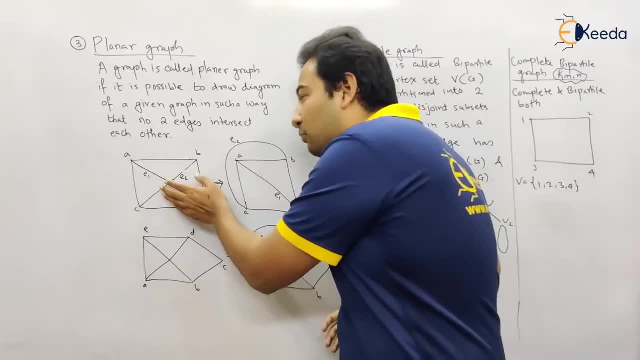 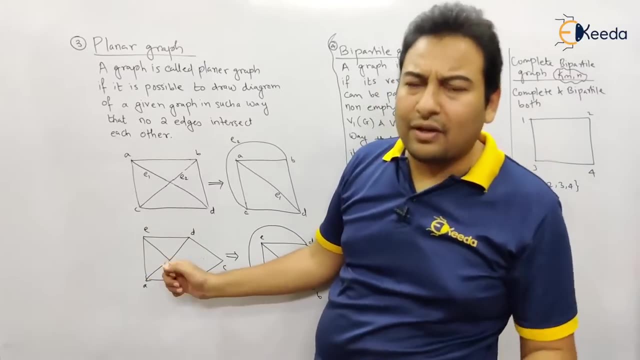 in a such a way that no two edges intersect each other. so if it is possible to draw in such a way that no two edges intersect each other, then it's a planar graph. again the same graph, again. one more graph here. is it a planar graph or not? first thought is not a planar graph, because they are. 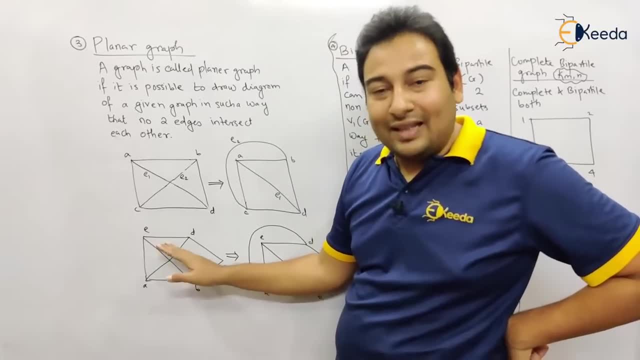 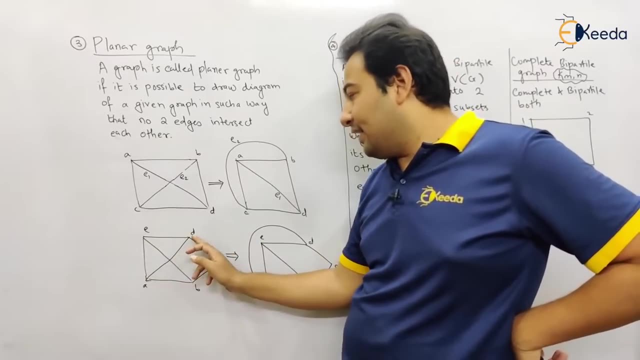 intersecting. but they are not intersecting because there is no connection here. this graph can be redrawn in such a way that this edges are not no more intersecting to each other, how this A- D you can redraw in such a way that so this is called a planar graph, or simply. 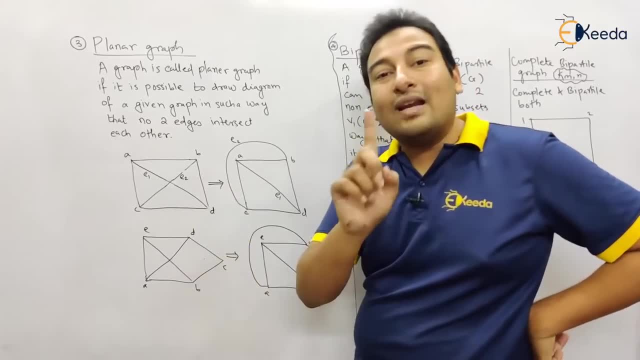 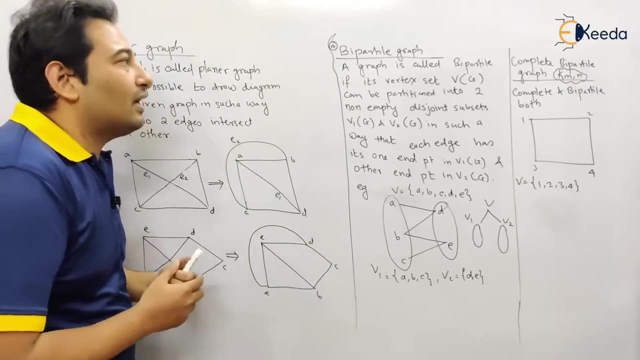 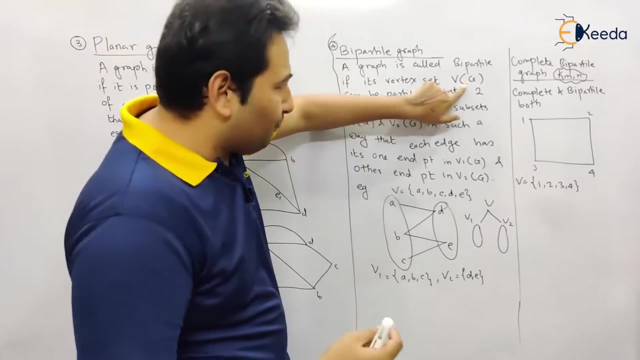 you should be able to represent a graph in one plane. that means there should not be any intersection of two edges. so this is planar graph. let us talk about the next graph, that is, bipartile graph. a graph is called bipartile if it's vertex set G V G, vertex V- G. if we are. 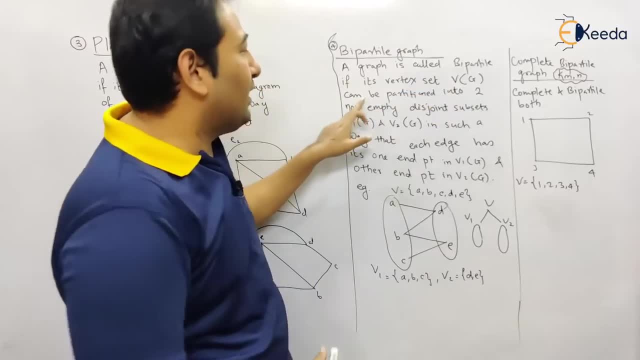 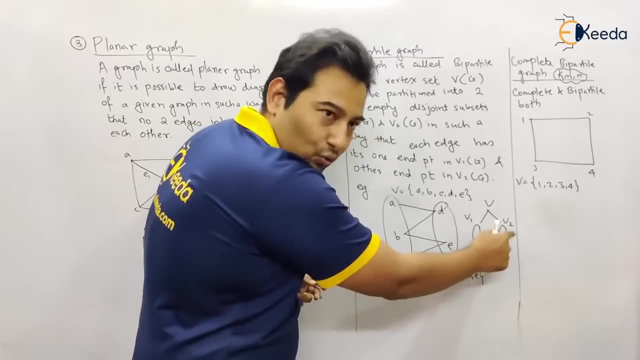 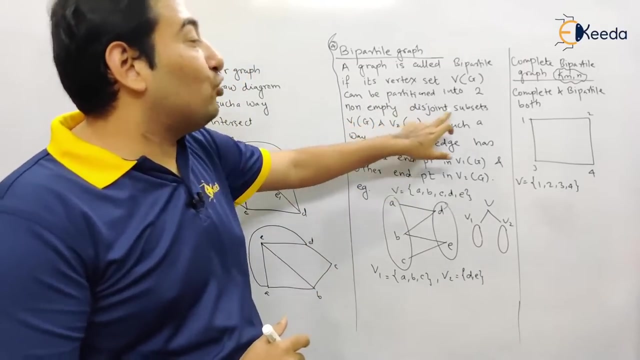 about this particular graph. there are five vertices: a, b, c, d, e can be partitioned into two non-empty disjoint subsets. so we we need to partition into v1 and v2 such that there are two conditions each edge. first of all, non-empty disjoint subsets, disjoint subsets. so what do you? 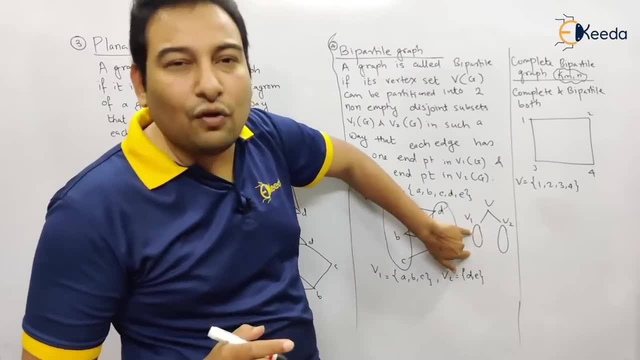 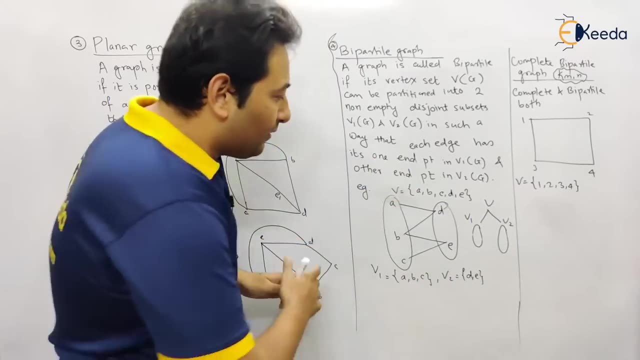 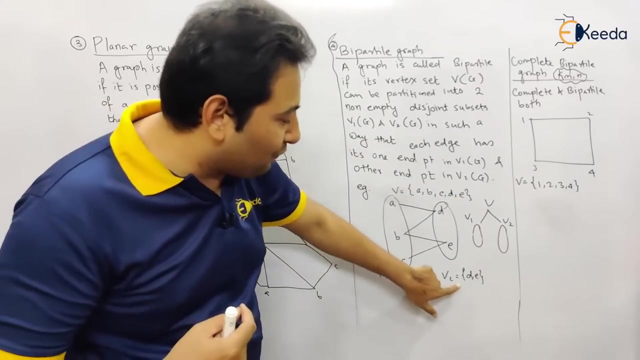 mean by disjoint subset. that means if we take intersection of v1 and v2, then it should be five. that means between v1 and v2 there should not be anything common. see here: we we have five vertices. we partition into two sets, v1 and v2, and they are disjoint sets because if you take 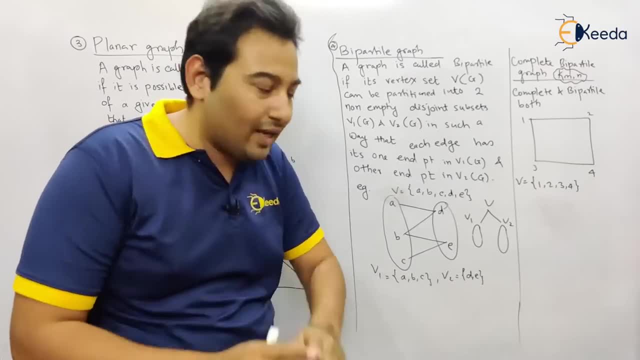 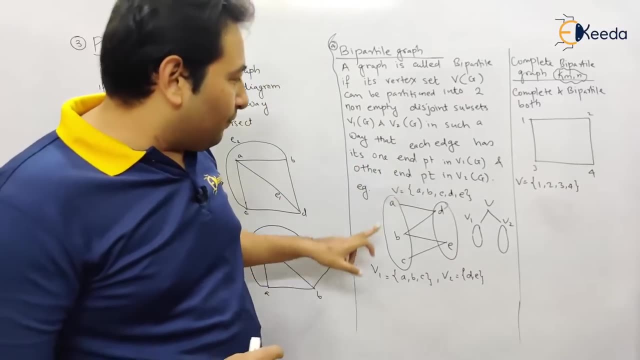 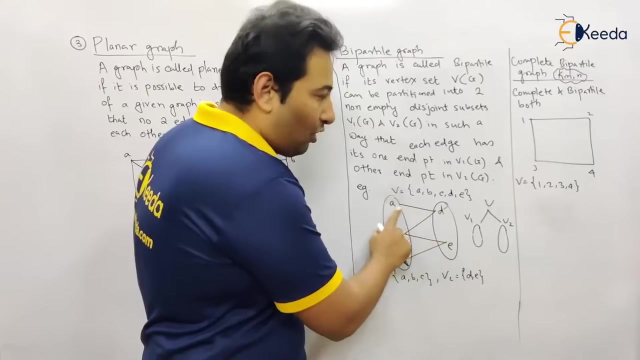 intersection of these two. there is nothing common or, in short, you can say: nothing common should be there between the two sets. and there is one more condition: one end point in v1g and the other point in v2g. every age, if we talk about this particular age, if it's, one endpoint is a and the other endpoint is d. 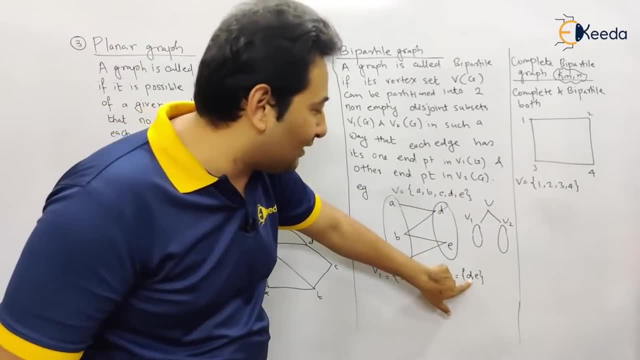 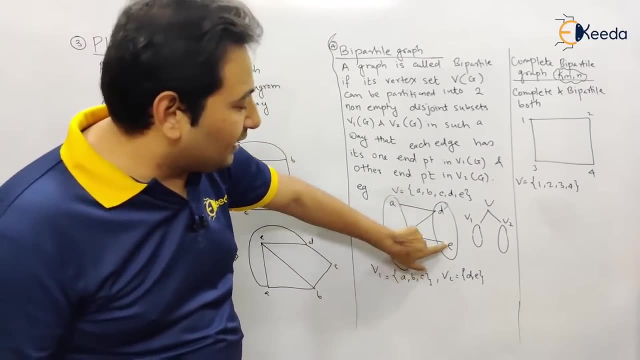 so a should be present in one set and d should be present in another set. for example, if we talk about this particular age, b is present here, d is present here, c is present here, e is present here. so these are the two condition. if these two conditions are satisfied, then the graph is: 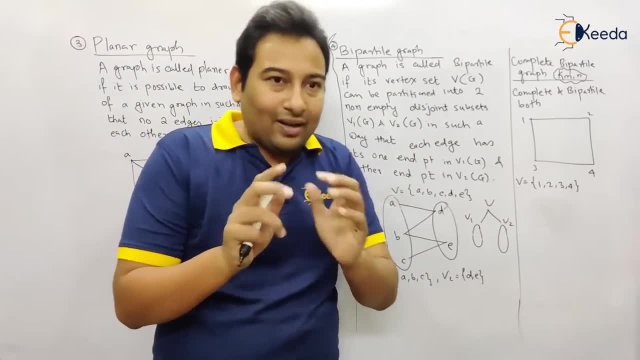 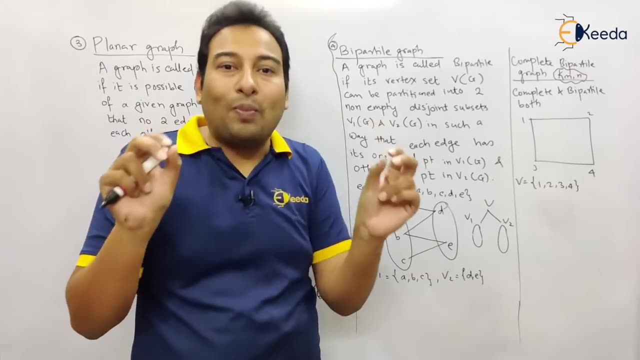 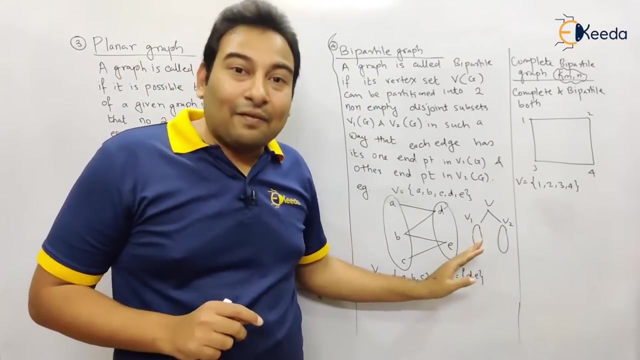 said to be bi-partile graph. are you clear with this? let me? let me repeat again. so there are two conditions. what is our aim? we want to partition v into two partitions, exactly two partition. therefore, it is called by: okay. so we want to partition v into two partitions. first of, 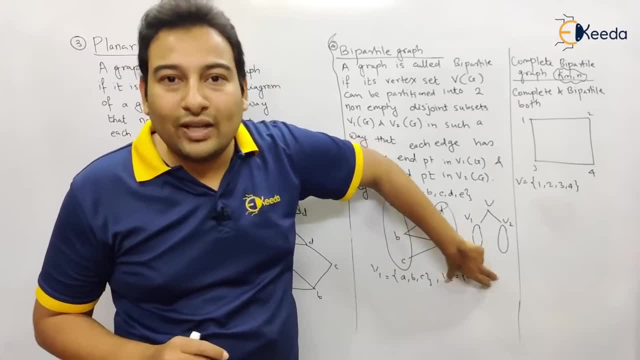 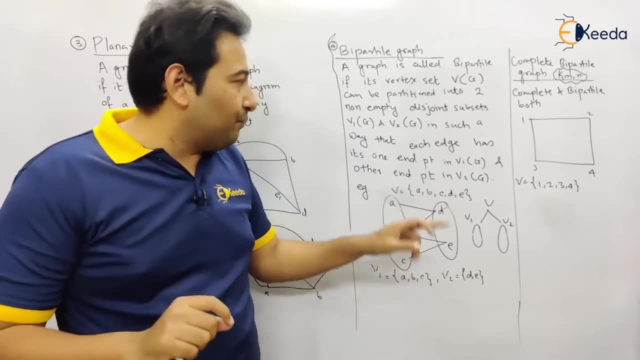 all, there should not be anything common both. if you take intersection, nothing should be common between the two partition. and the second condition is, if we consider any age, one point should be in this partition and the other point should be in this partition. are you clear? or the second point? 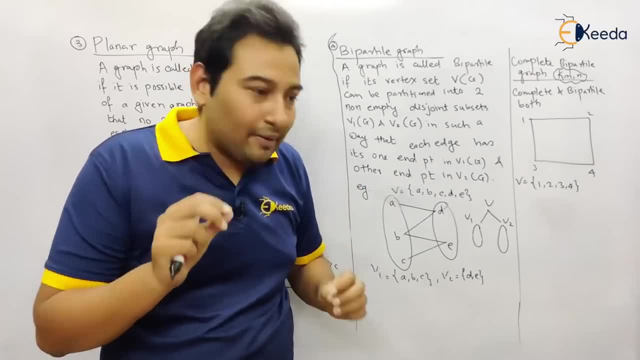 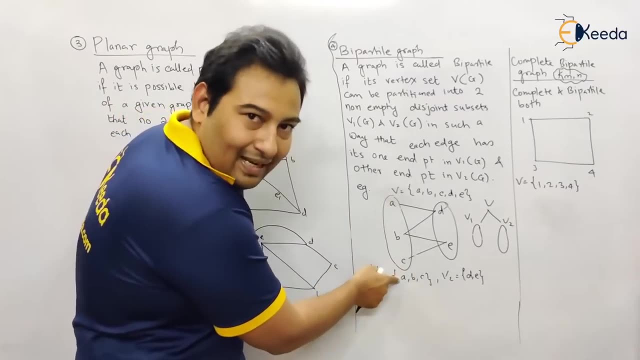 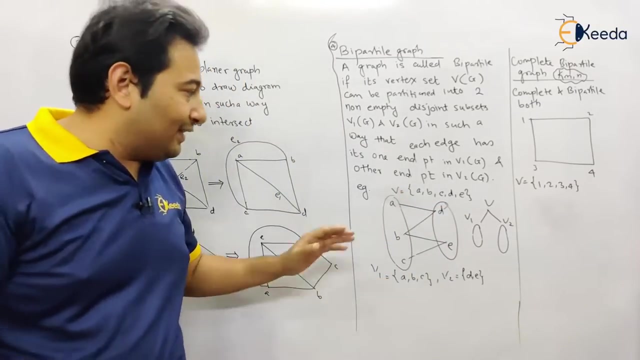 you can simply say there should not be any age between the vertices of the same set. that means here a, b, c are the vertices of this particular set. there is no age between this, because age is from this set to this set. there cannot be age between this set. then it is called your bi-partile graph. 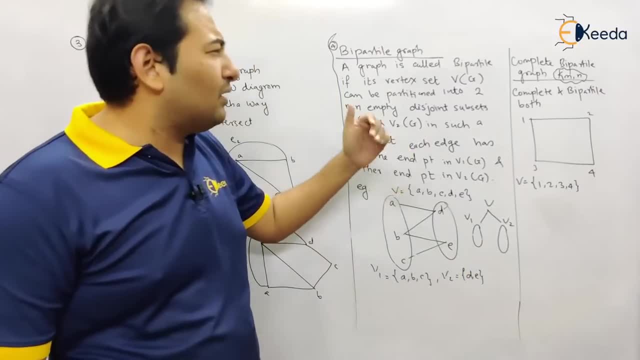 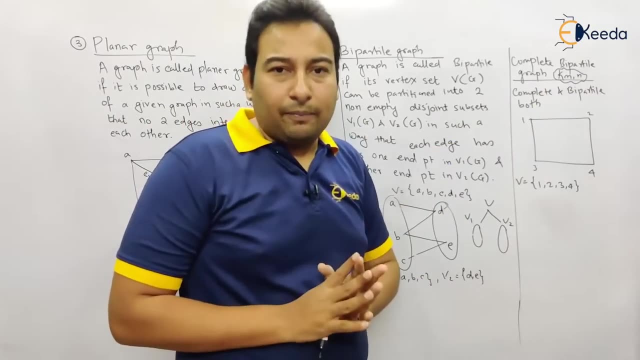 now. the next is complete bi-partile graph. complete bi-partile graph, you can say, is one more variation of bi-partile graph. it's very simple: it should be complete as well as bi-partile. that's it. first of all, please tell me how many vertices are there? 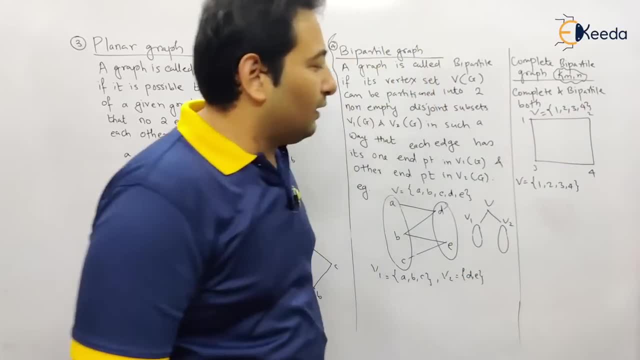 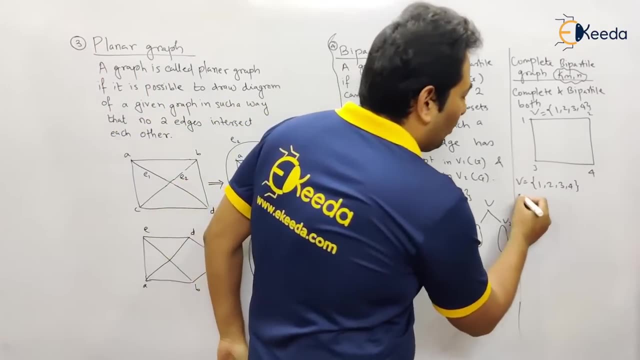 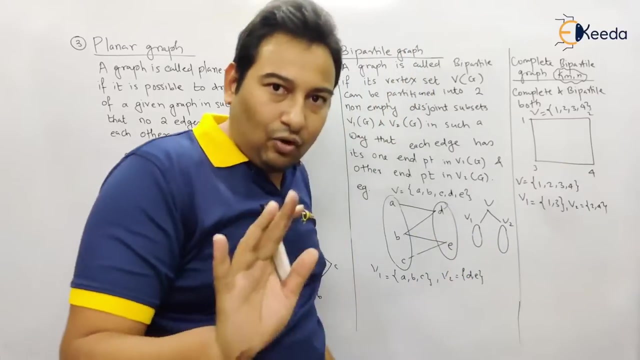 one, two, three, four. i want to. i want to by partition it. i want to convert it into two partitions. so what are the possible? what are the options? see here, one, three, and let's say v2 is equal to two, four. now i have two partition. first of all, let us take the condition first. 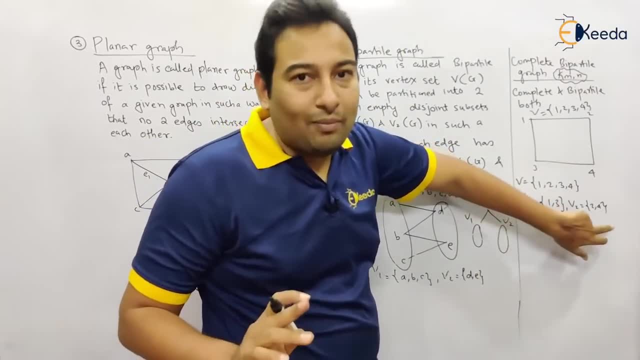 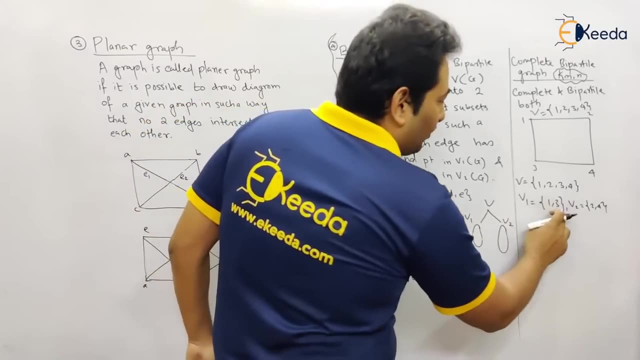 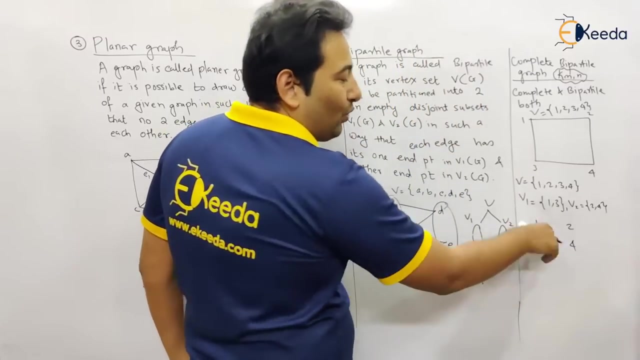 of all, there are two partitions. nothing common in them, if you take you intersection. there is nothing common. so first condition is satisfied and let's, let's draw a graph with the help of this partition. so there are one and three, and two on four, one and three, one in one partition, two and four in the other partition. 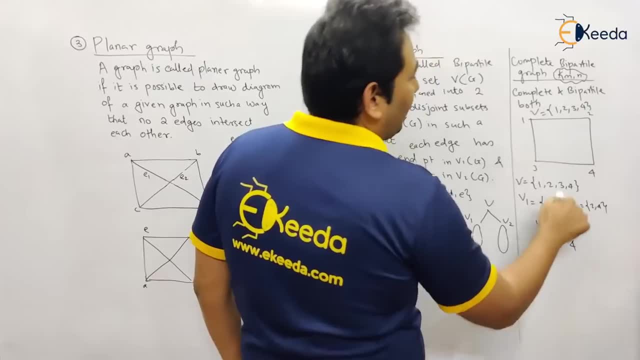 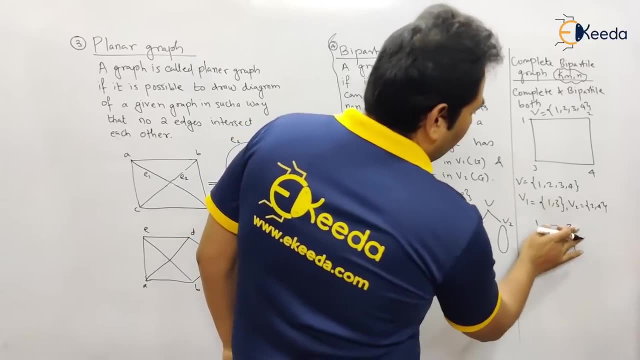 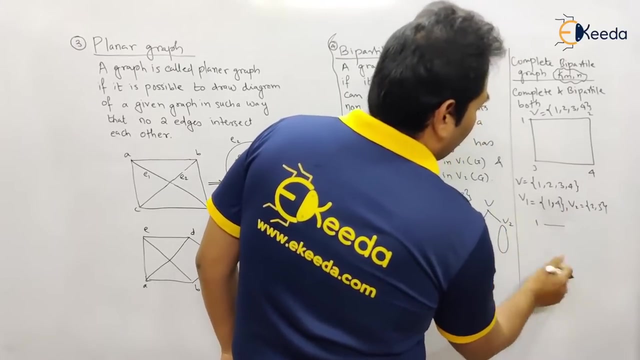 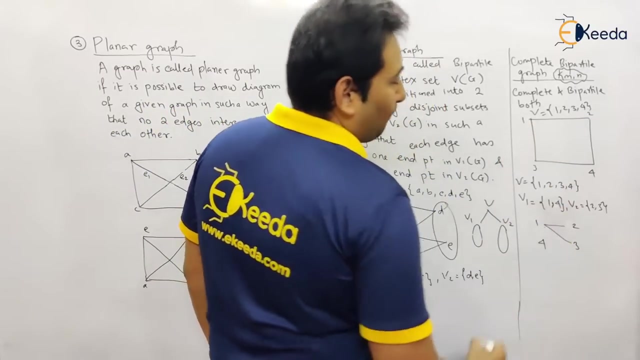 so what is the age? so age is between one to two. so perfectly fine, then it is between one to three, c here let's make it one, four and two, three. now, one, four will come here, two and three will come here. so, but age is between one, two and one, three. see here. next, where is the next age? it's between: 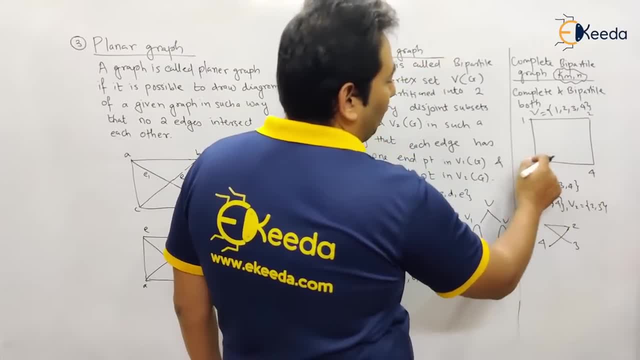 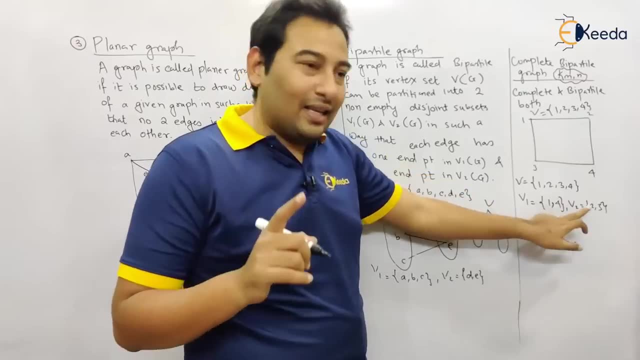 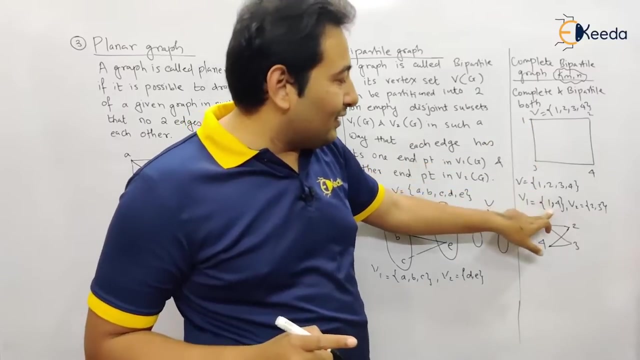 four, two. see here between four, two and four, three, one and four in one set, two and three in the other set. there is nothing common in between if we talk about this particular age. the starting point is in the set, ending point two is on the other set. 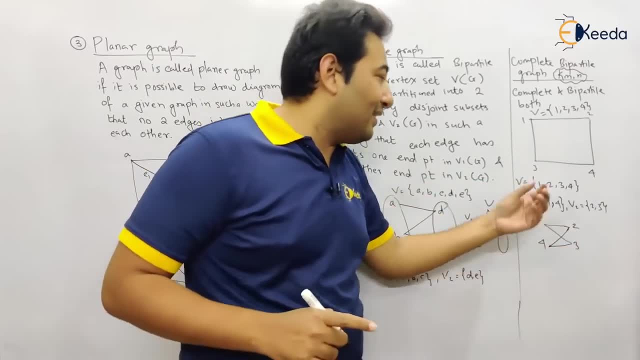 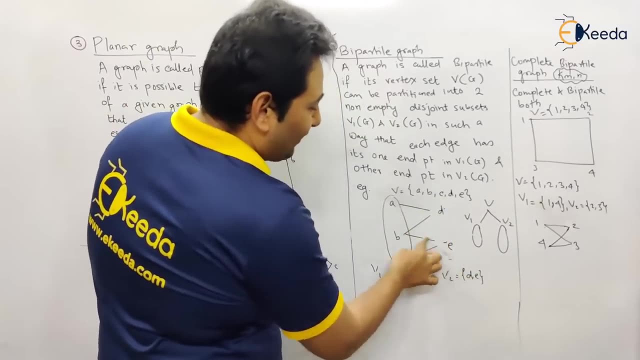 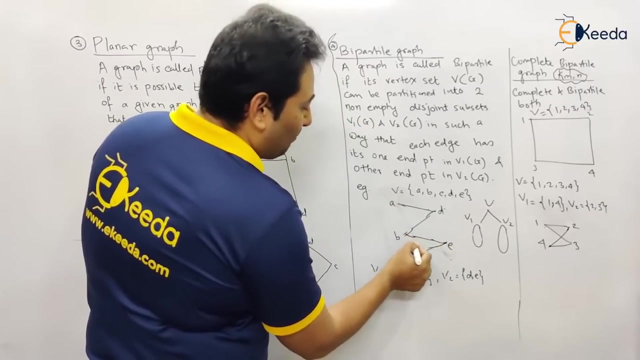 starting point three is one in one set, ending point four in other set. so this is basically satisfying all the condition. so this is circle i just made to show that it's in one set. this is actually your graph. please tell me, is this clear? so complete bi-partile graph means it. 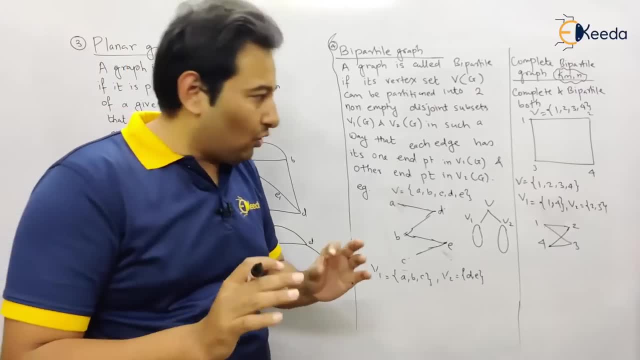 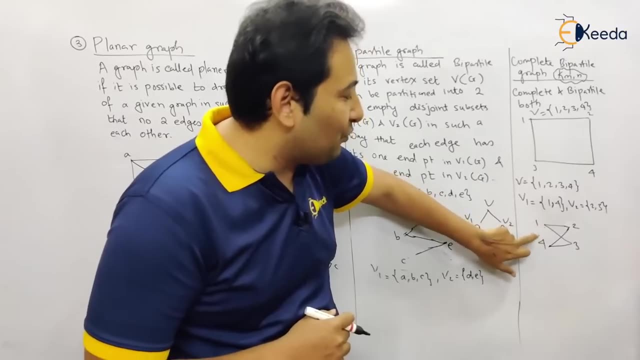 should be complete, and the next is it should be bipedal. first of all, there cannot be any uh age between the vertex of the same set. that means between one and four. you cannot have a word, you cannot have age. so that is exception. but complete means. 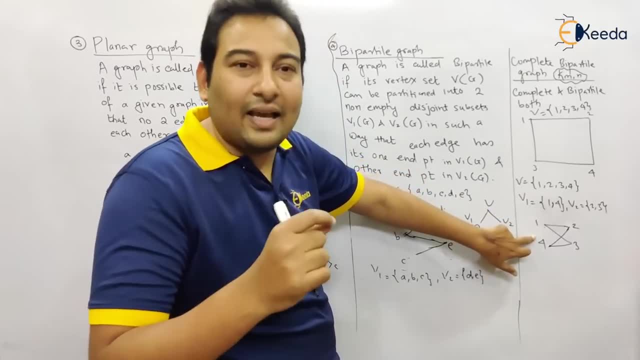 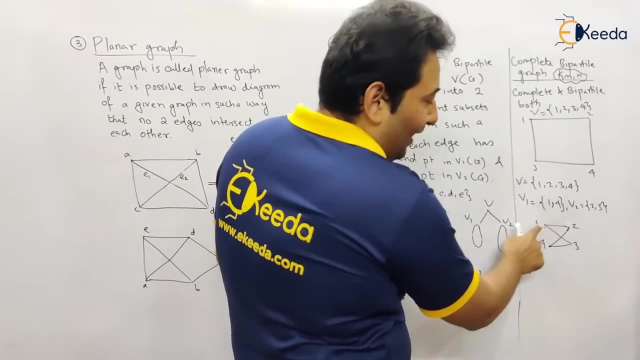 vertex of one set must have connection to every other vertex of the next other set. that means here: so from one, what are the possibilities? two and three: from one, it is connected to both the vertices. from four: it is connected to both the vertices. therefore, it is a complete graph for. 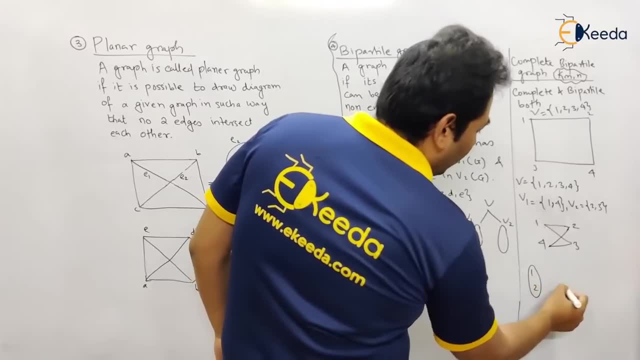 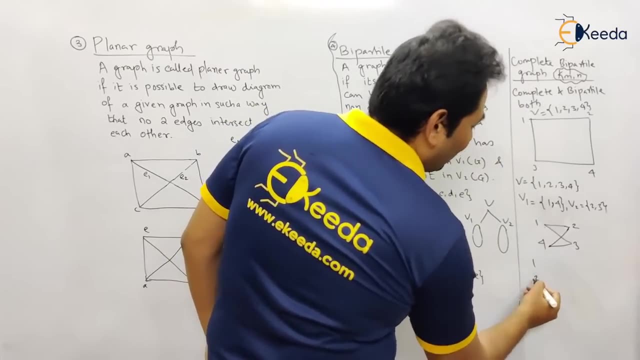 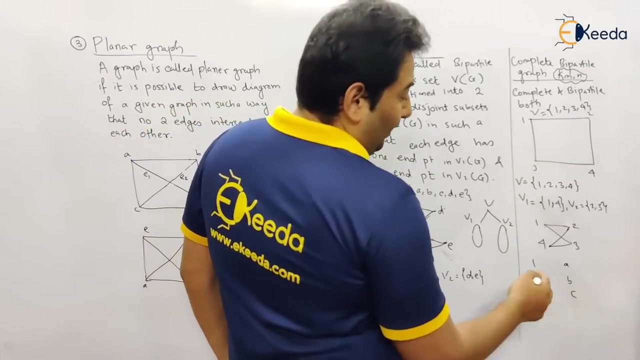 example, let's say uh, if i'll say there are two points here and let's say there are three points here, now if it's a complete graph, first of all, see. so in one set i'm having one, two element. in the second set i'm having a b, c element. so what is a complete graph? and by uh, by partile c here, 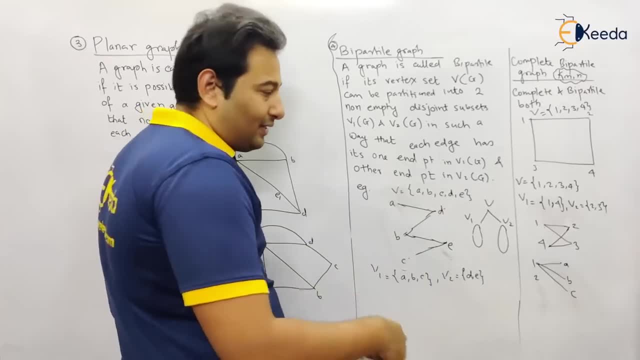 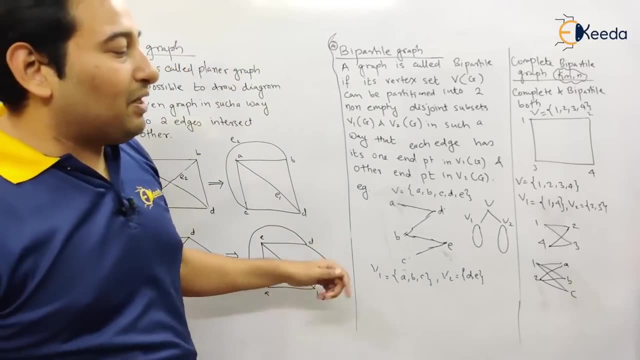 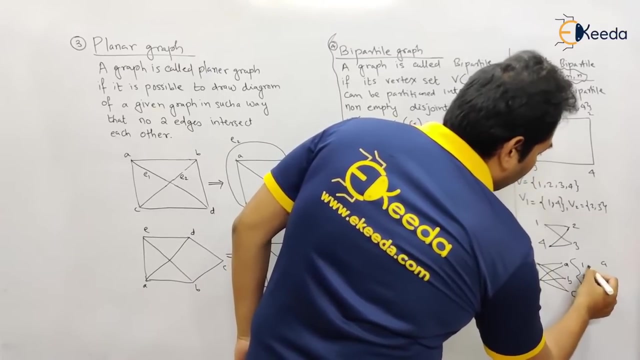 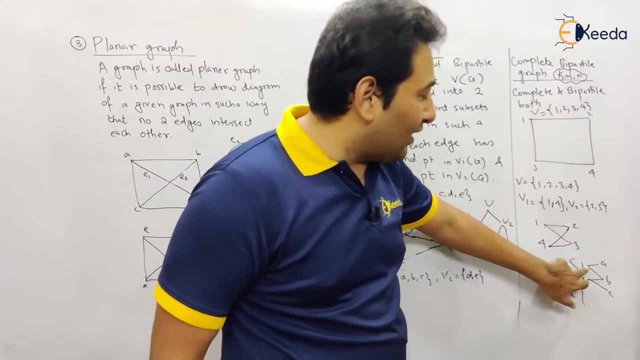 one is connected to all the elements of the or the vertices of the other set. likewise, two is connected to all the vertices of the other set. so this is, you can say, complete bipedal graph. see just for bipedal, it is enough. this is also bipedal where one is connect. one is not connected to c. it is bipedal. 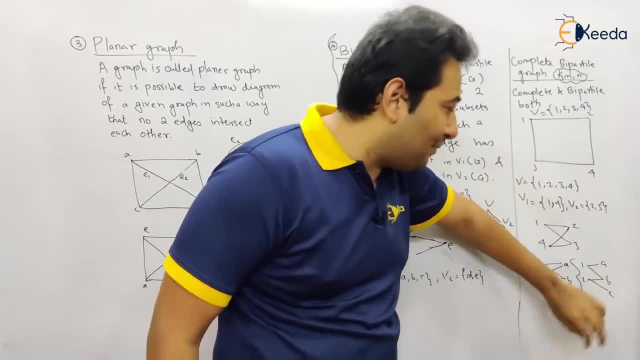 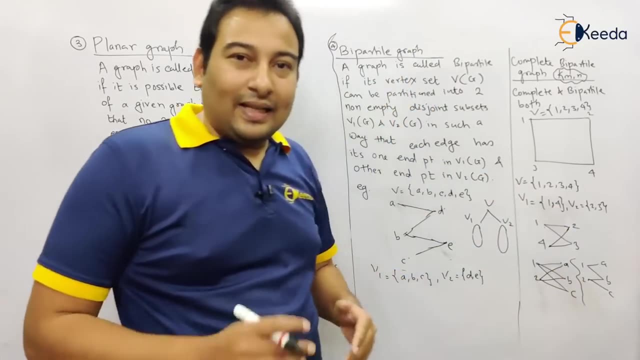 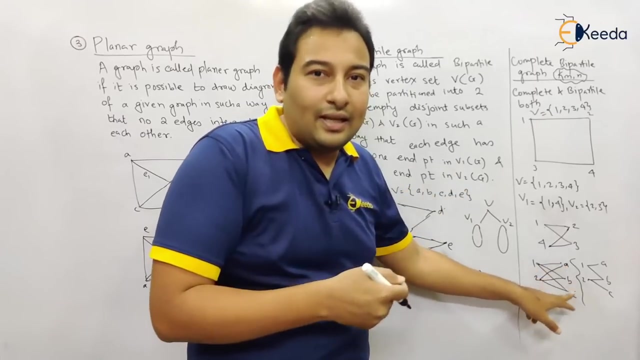 in first set there will be one, two elements. in the second set there will be abc element and there is no link between the sets of the same vertices but it for complete bipedal, it to be a connection between each vertex of the set one to the all the vertices of the uh set two. i. 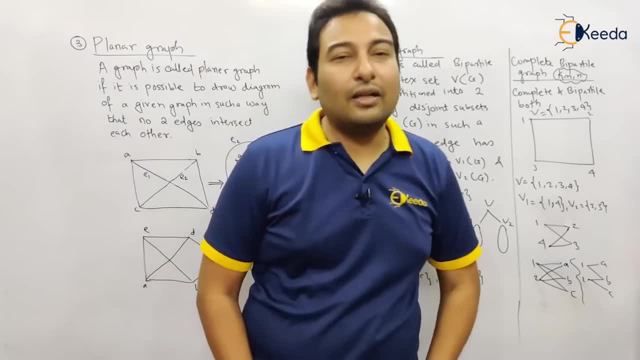 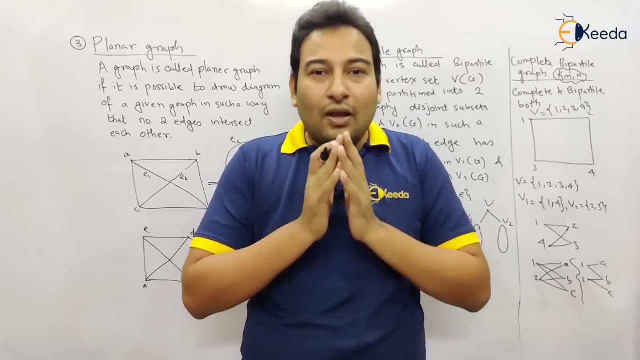 hope this is clear. bipedal graph and complete bipedal graph. so these are the different types of graphs. so in this video we discussed: uh, what is graph? what are the different types of graph? in the next videos we'll discuss few more concepts. we're done with the video. hope you understood, thank you.